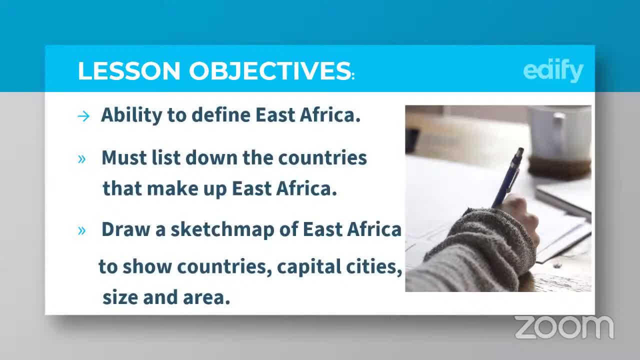 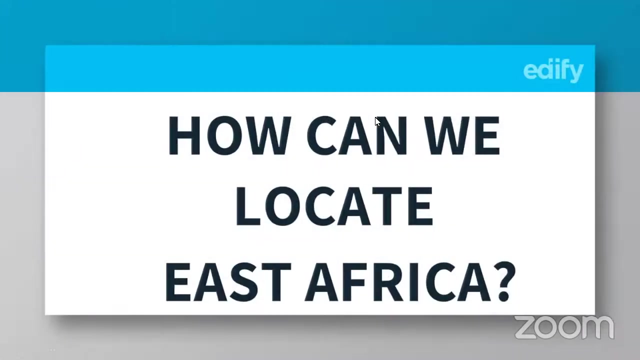 Then you should be able to list down the countries that make up East Africa, And then I want you to be able to draw a sketch map of East Africa that shows the countries and the capital cities and how it is- Okay, Distributed as far as area is concerned. That said, how can we locate East Africa? I need someone. When you talk of East Africa, what comes to your mind, Priscilla? 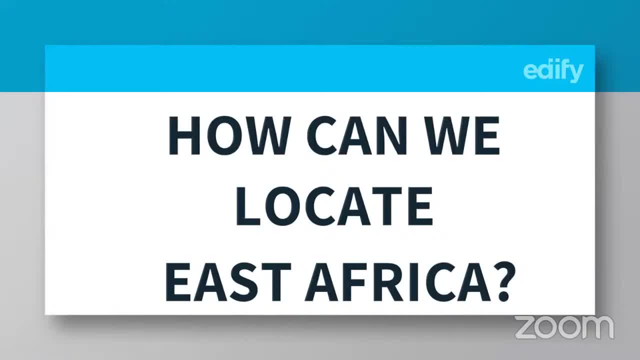 When I talk of East Africa, what comes to your mind? Uganda, Kenya, Tanzania, Do you think of? When I talk of East Africa, what comes to your mind? You think of Uganda. That is Opoi talking, Opoi. you think of Uganda, Okay. 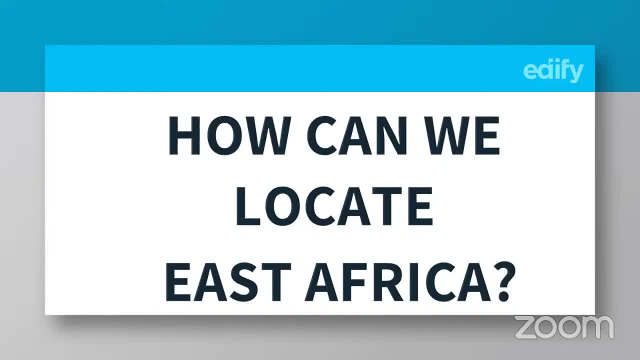 Someone is thinking. Mogesha in the chat is saying he thinks of the eastern direction. Beautiful Olum. when I say East Africa, what comes to your mind There is East And Africa. Shadiq is saying countries in the eastern part of Africa. Shadiq, that is a beautiful idea. 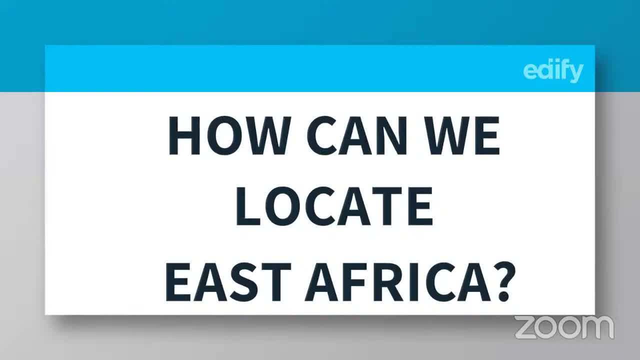 Shadiq, when he hears East Africa, he thinks of countries in the eastern part of Africa. Hagad, Malay is saying Uganda, Kenya and more. Okay, I love the fact that you're all on track, Or both. When I talk of East Africa, what comes to your mind? 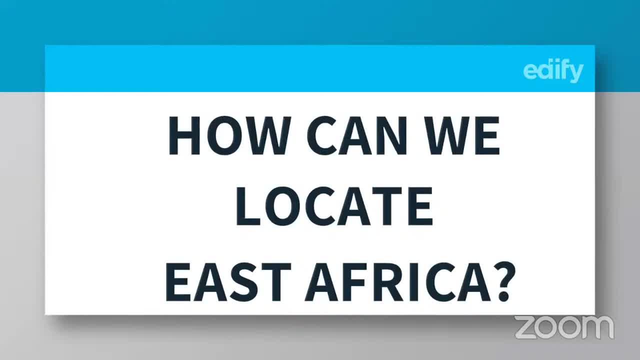 Alvin And Mogesha in the chat. Aina, Mogesha, thank you. He's saying, I think, of the eastern side of Africa. Alvin, you're very right. So today's lesson, you're going to analyze the eastern side of Africa. 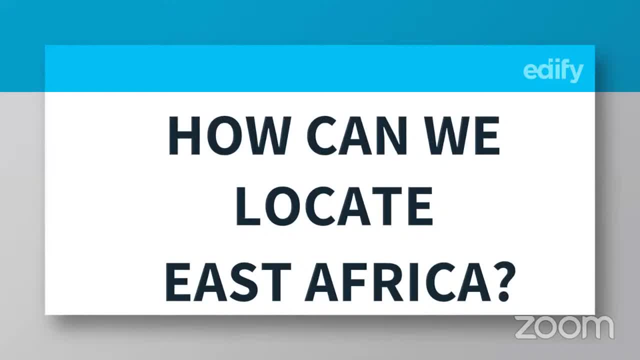 Prosperous is saying countries in East Africa. So we are going to look at the eastern region. Thank you, Nansam. but the eastern region of Africa, Martha, is saying the East African community. All your ideas are very right. So, meaning we can locate East Africa And I'm giving you that East Africa is basically we're talking about the countries in the eastern region of Africa. 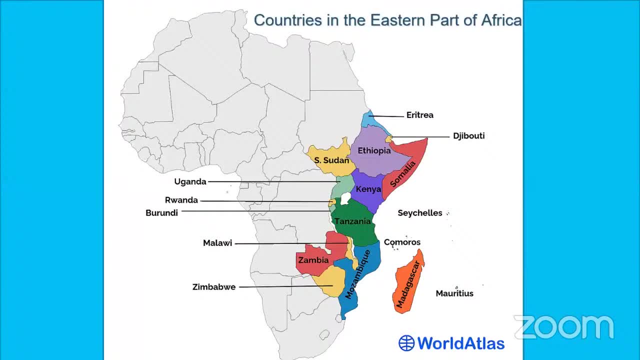 So there we are. If this is direction and you put your campus direction on this map, okay, Okay, If I'm to have my campus direction on this map, if I'm to draw it Somewhere, I'm to draw my campus, then I draw my campus direction. sorry, the line is not straight. so, which is the east, which is the west, which is the north, which is the south? 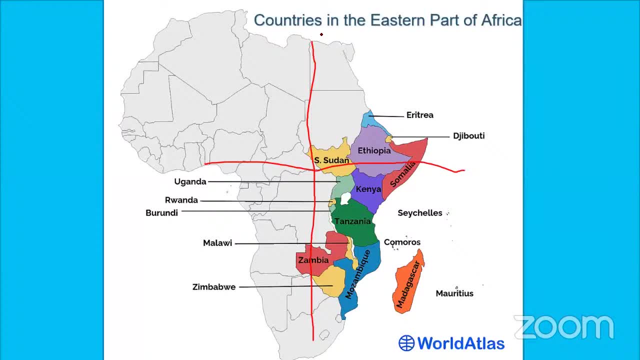 So I'm going to have my north up, Then I'll have my south- Forgive my poor handwriting- Then I'm going to have. if you have problems locating east and west, just write the word we. We are eating we such that where the W is is the west. 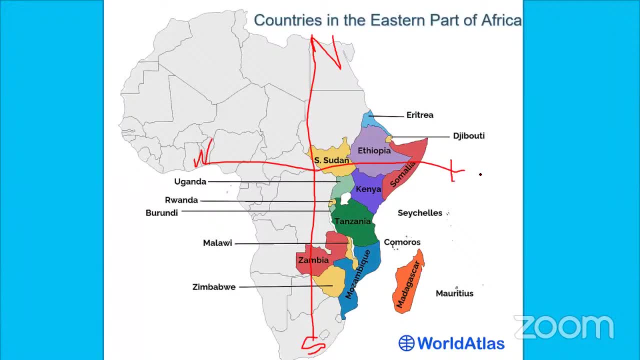 And where the E is is the north, And where the E is is the east, Is the east Is the east. So we are going to look at countries in the eastern part of Africa. Are we together? So which countries are you seeing? 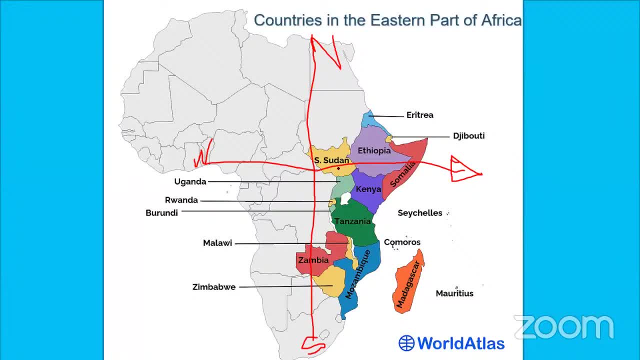 Because I think we can further divide these countries into. there is northeast. okay, Look at those countries. So I have the northeast. Okay, Okay, Then we shall have countries in the south-east as well. So we have the north-east. 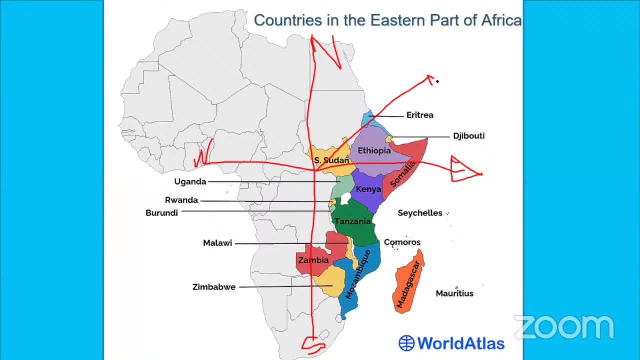 Then we shall have the countries in the south-east as well, Then, so, Then. so Look, north-eeast is the east, so we shall have countries in the south, is so. i want us to group this, is this africa, into three. we have those in the east, we have those in the northeast and those in the south, is so. 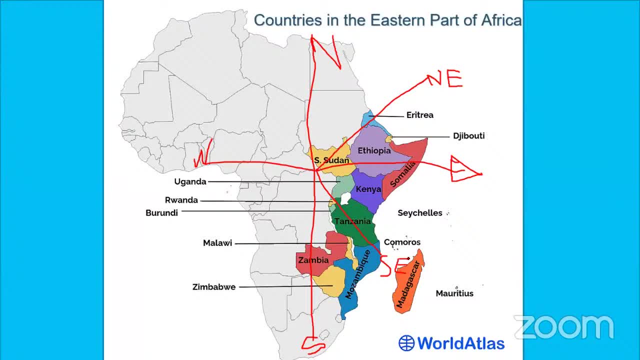 what are the countries in the north east of africa? so if this is my african continent, the eastern part generally is the one that has countries that are shaded. i hope you're following now. what are the countries in the north east? countries in the northeast, zack, zack, say something. 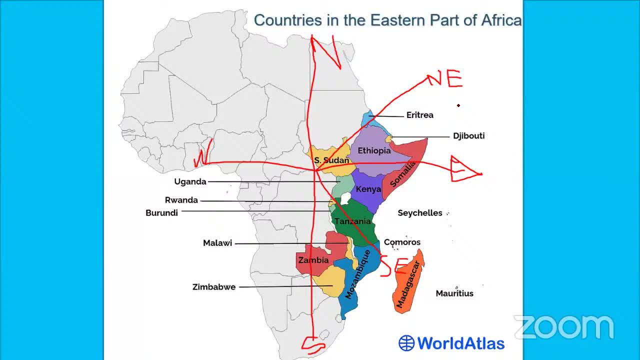 what are the countries in the northeast? yes, zack, south sudan, itria, there is south south sudan, the south sudan, okay. eritrea, there is eritrea, and somalia, and somalia, okay. which other name can we give these countries in the northeast? 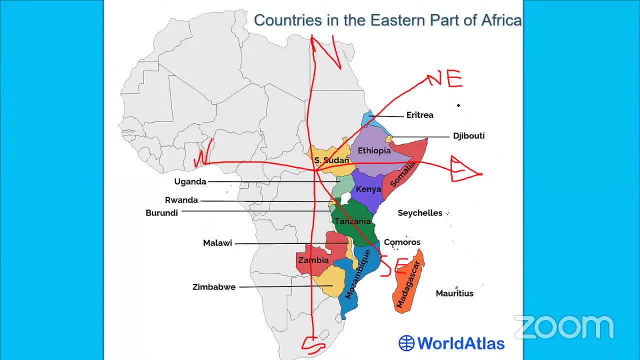 countries in the horn of africa beautiful. so those are the countries in the horn of africa. the horn of africa is that part we are seeing. okay, countries around there are the ones you're calling the countries in the horn of africa. what are the countries in the eastern parts? 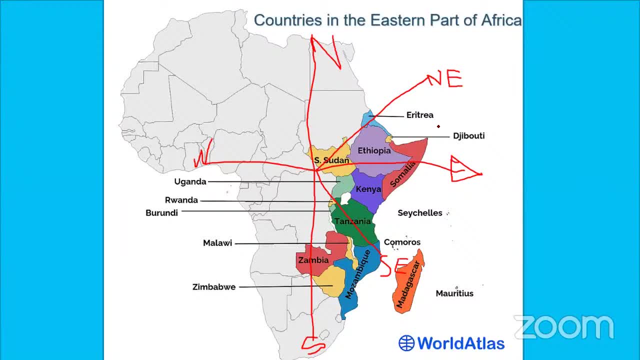 africa, directly in the east of africa. tessa, tessa, say something. uganda, there is kenya and tanzania, tanzania, somalia. somalia is also in the east, can you see? hmm, i see it like it's a. in that it's maybe my campus direction was not really accurate, but if you were to look, if this 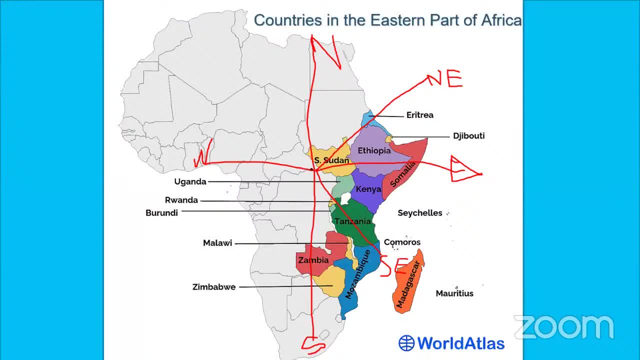 is my east, directly the east. if i put it a little bit lower, it would be uganda, kenya, tanzania. uh-huh, we have randa and burundi. they're the countries in. that is what is common about these countries. what do you think is common about these countries? 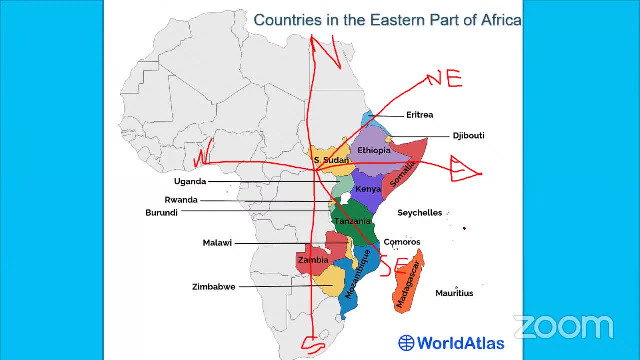 yes, Uganda, Kenya, Tanzania, Burundi, Rwanda and South Sudan as well. I think they are all in the East African community. beautiful, they are all in the East African community. so we have grouped the Eastern countries of Africa as those in the Horn. we have now those in the East African. 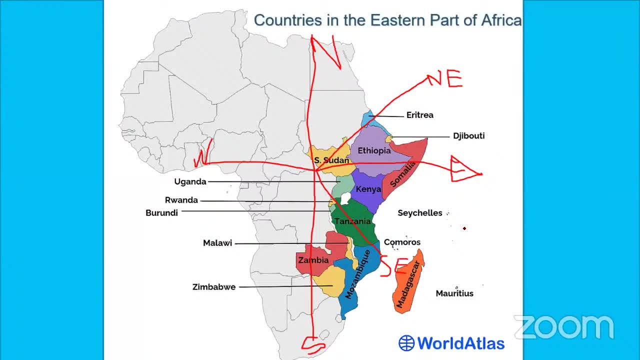 community, amazing. what about the countries in the South East Africa? South East Africa, which countries are we seeing? Tina say something. countries in the South East Africa. let me read through the chat. the hands are too many. yes, Tina, commerce, search and use. Mozambique, Africa, Zanzibar. 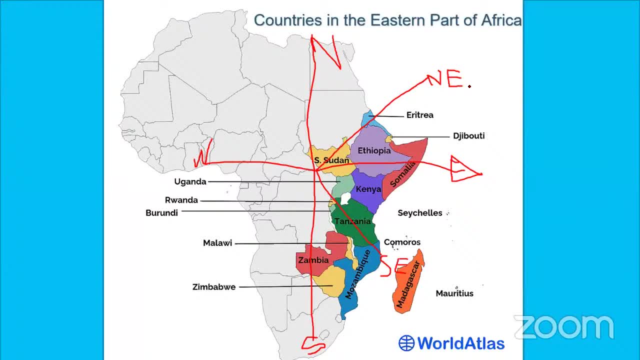 Zanzibar. so in the South East we have Mozambique, Madagascar, Zanzibar. is there a Zanzibar anywhere? Tina, are you lying to us? is there a Zanzibar? no, can someone help Tina? who is helping Tina? Joseph Stephen, Joseph Stephen. 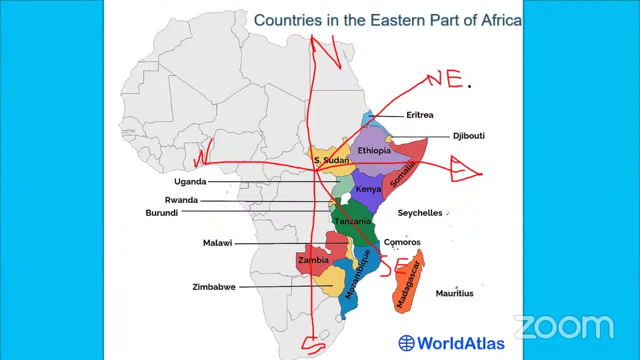 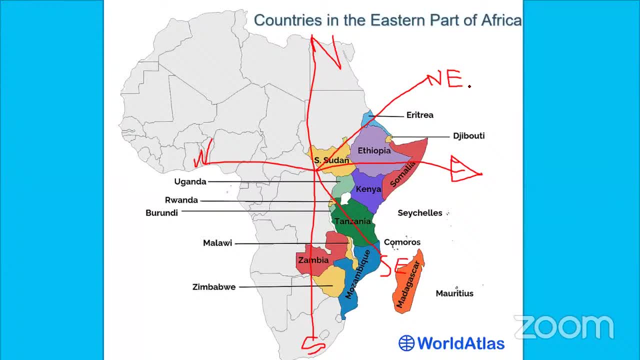 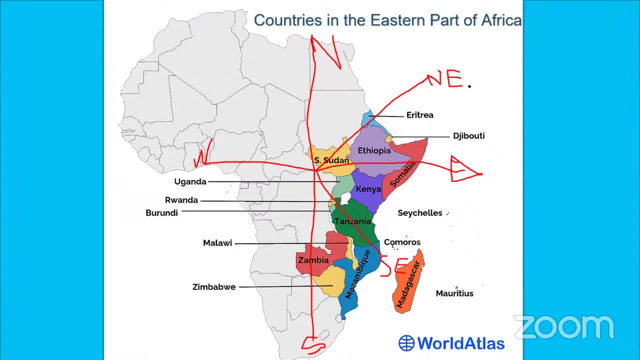 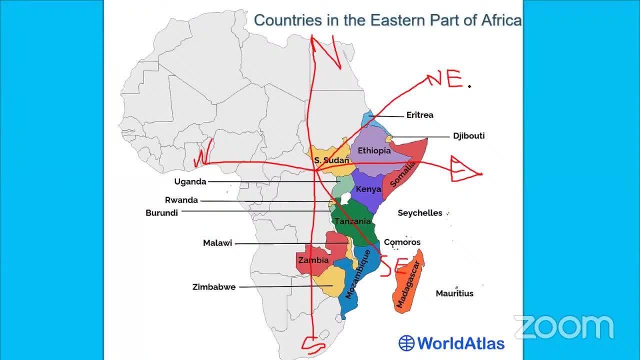 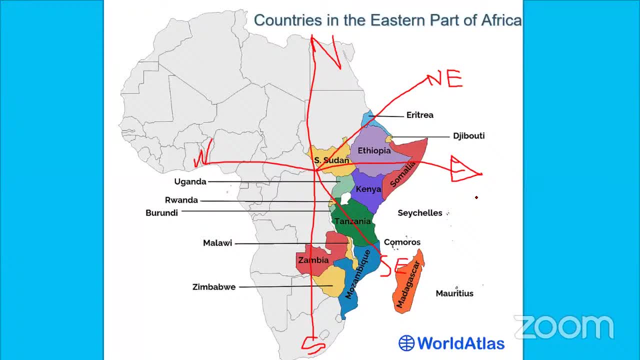 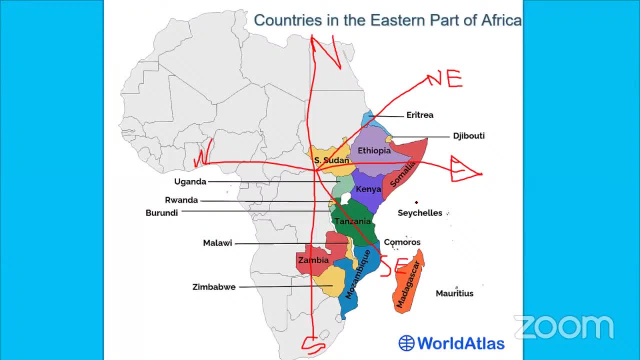 in the indian ocean. we have seashells, we have comoros, we have mauritius. there's reunion down here, island country. amazing, there are countries found in the islands of east, the eastern part of africa. so basically we have grouped the eastern countries into, i think, four. 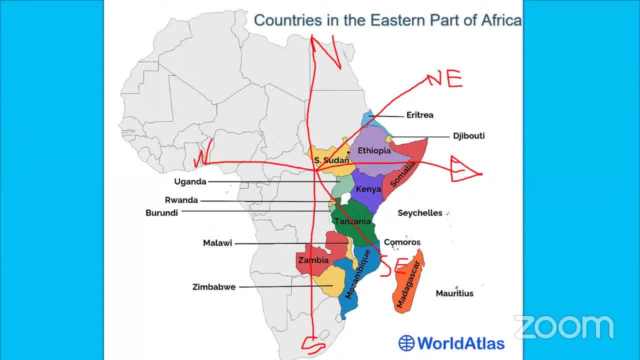 none. so we said we have those in the horn of africa. we have those in the horn of africa where we looked at eritrea, djibouti, ethiopian, somalia. then we have those in the east african community, and so then you have looked at those in the southeast of. 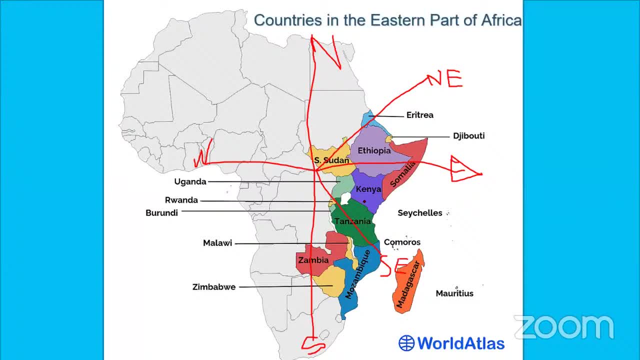 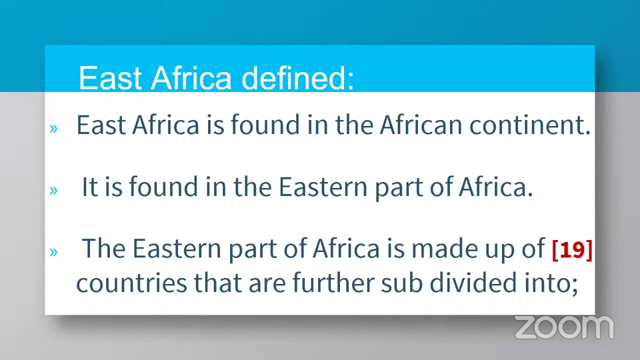 africa and then finally, those in the island region: seychelles, comoros, madagascar, mauritius and reunion- good, so let's group them. so east africa- if i've defined east africa, we can. i did not say this is east africa- is formed in the african continent. do you believe that? 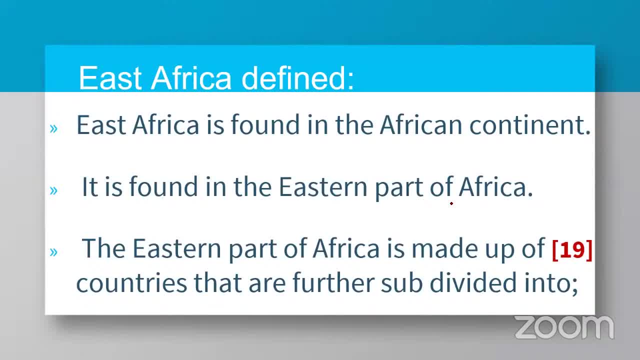 if you're done raising your hand, please put it down, because you're confusing me. i feel you have a lot to say. east africa is from the eastern part of africa and it is it has these countries that we have further divided into four island countries. thank you, 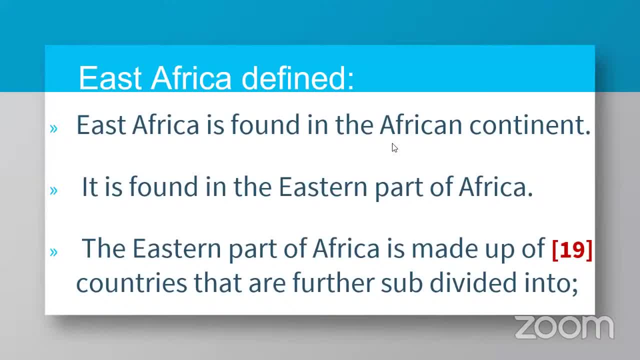 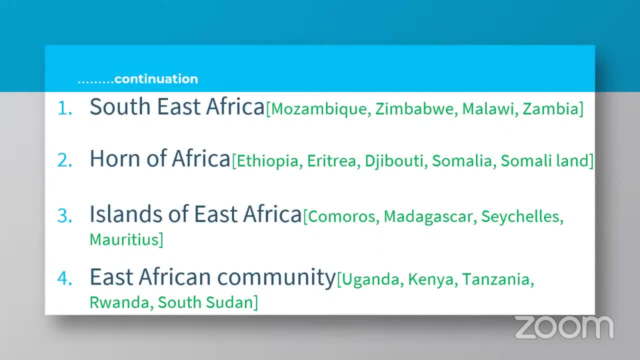 four island countries, thank you So, which we have grouped into four, where we've looked at those in the southeast, which included Mozambique, Zimbabwe, Malawi. Then we have those in the Horn of Africa, that was, Ethiopia, Eritrea and Djibouti. 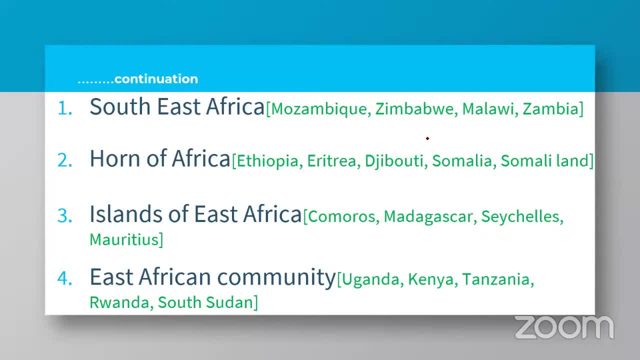 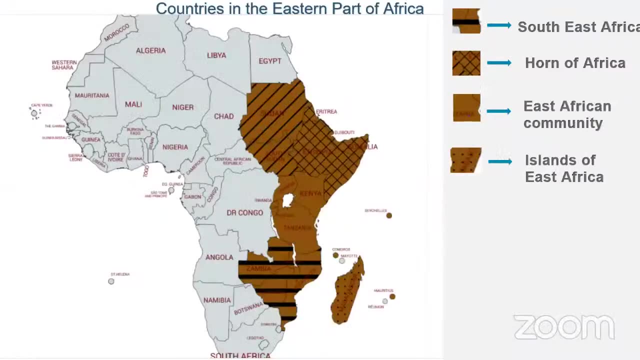 Then we have those that are the islands and then those that belong to the East African community. Okay, I like your contributions Very right, So let's continue Now. these are the groupings we have given in our discussion that we've grouped the countries in East Africa into four. 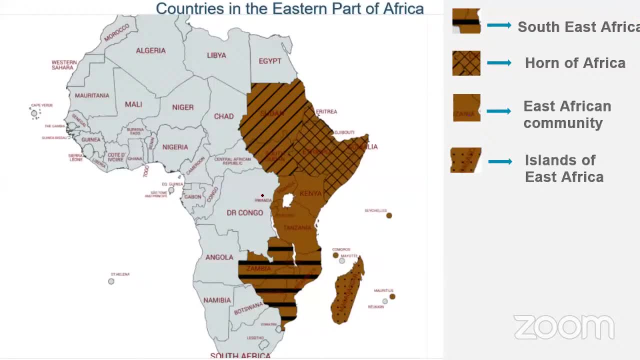 Those are in the southeast. which are these ones here, Those in the southeast? I think you can see on my key, we have those in the Horn of Africa: Eritrea, Djibouti, Somalia, Ethiopia. Then we have those that are in the East African community. 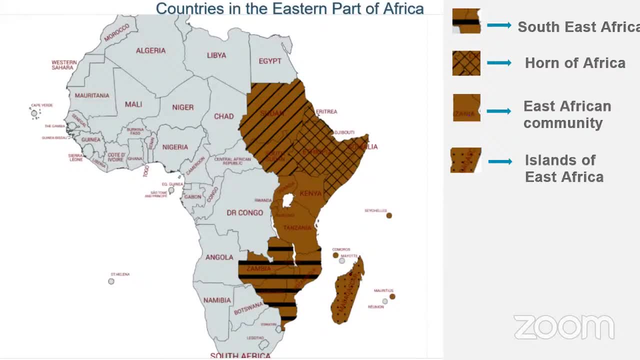 You can see the plain brown ones as well as those in the islands Seychelles, Comoros, Madagascar, Mauritius and Réunion. Any questions up to that point or you're understanding. No, thank you, I'm good, thank you. 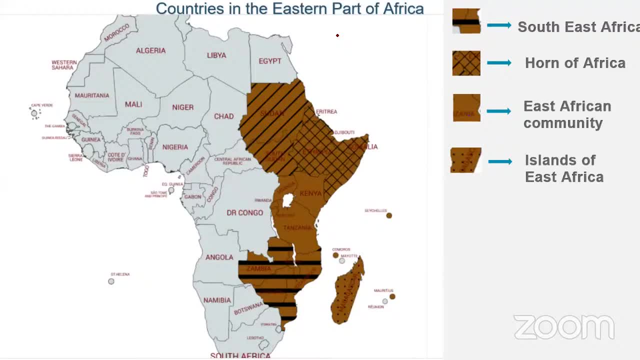 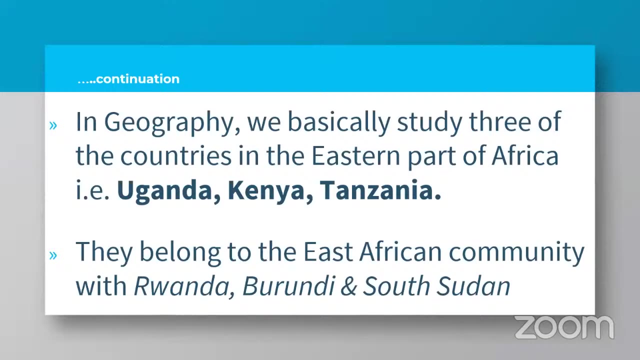 Someone is saying they're checking the classroom. I even marked work yesterday, treasure, You could be checking in the wrong classroom. Yeah, But we shall look at that later. Okay, So in geography especially so, we have looked at the eastern countries in the eastern part of Africa. 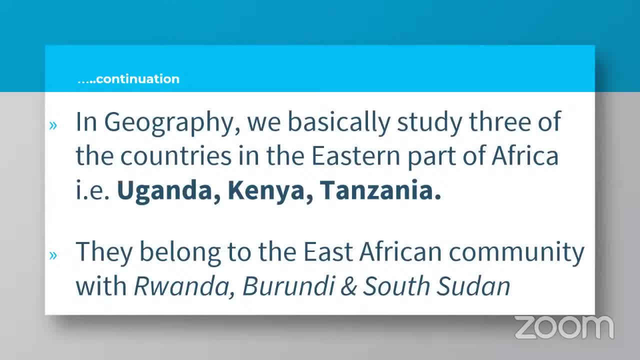 You would be confused. You'd confuse East Africa and countries in the eastern part of Africa. They are all in the eastern part of Africa. Africa is the large continent, and then those countries that are found in the east are the ones you're calling East Africa. 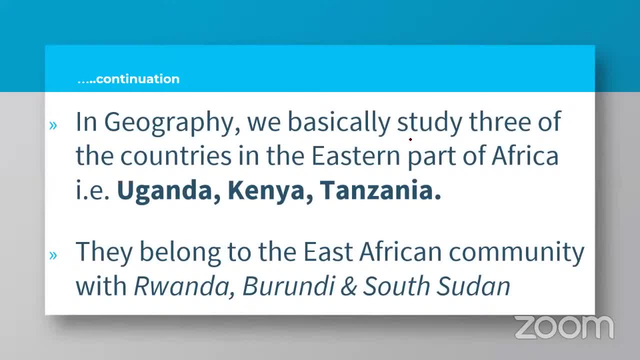 But in geography we basically study. We study the topology, we study the temperature, We study the temperature, We study the weather, And then we have the… three countries. in our geography lesson we basically study three countries, that is, uganda, kenya and tanzania, and what is common about these countries is that they all belong to the east. 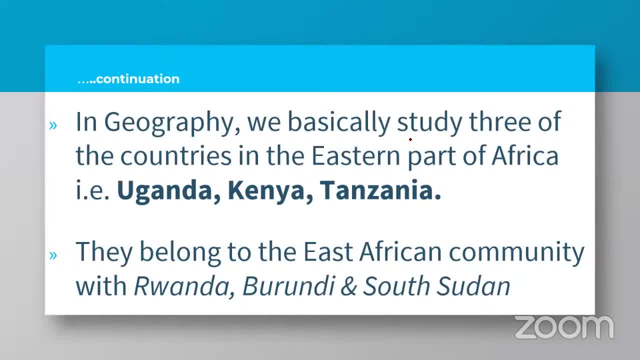 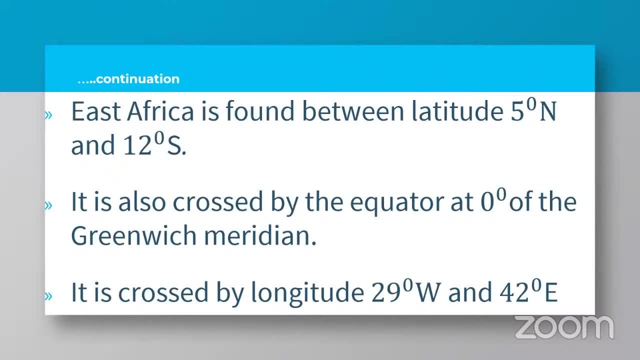 african community, like someone noted. okay, and that includes randham, rooney and sudan. okay then, if i'm to give latitudes, i don't know if someone knows the difference between latitudes and longitudes. i want someone to give me the difference between a latitude and the long. 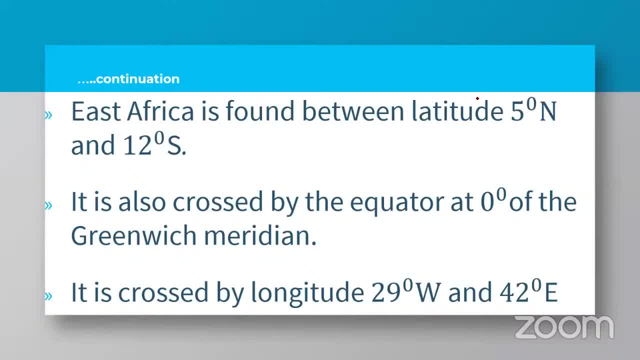 yes or both, or both. your hand is up. what is the difference between latitudes and long sheets? latitudes are imaginary lines drawn on the map running from north to, from east to west, from east to west, while long dudes are imaginary lines drawn on a map running. 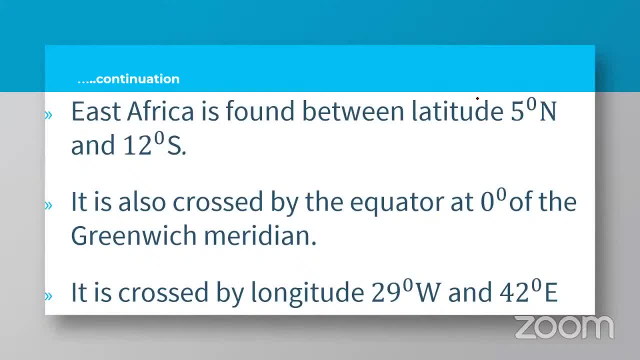 from north to south of the globe, beautiful. so east africa also has lines, those imaginary lines crossing, running from east to west. okay, i think if you're to note in my notes there is a mistake, this is the wrong way. i don't. so, found between latitudes five degrees north. and so isn't this supposed to be a long food. this is supposed to be long two, five degrees north, so we shall cancel this right. so north to south, those are long Tuesdays. east west, those are north, so south, those are long Tuesdays. east west, those are. 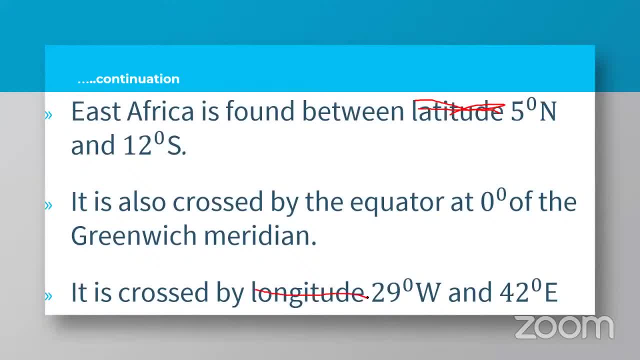 latitude. okay, so it's. africa is also crossed by latitudes and longitude. so we have longitudes five degrees north and 12 degrees south, whereas latitude 29 degrees west and 45 degrees, and then there is a major latitude line that crosses east africa, and that is the equator. okay, 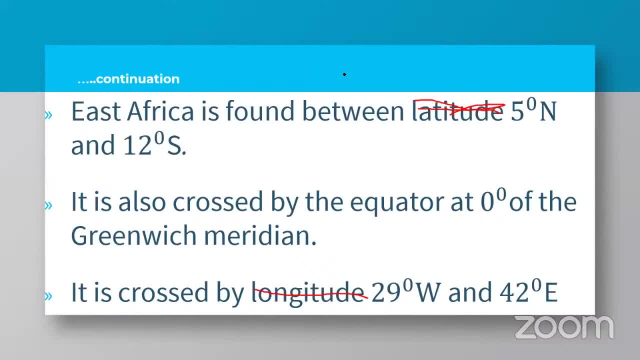 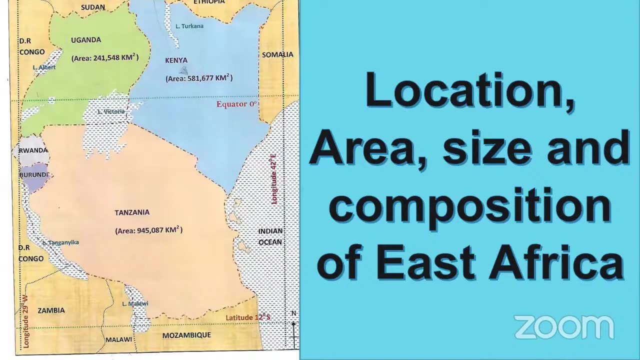 we are going to continue and look at how east africa actually looks like. this is where we are now. okay, this is east africa. we are looking at latitudes: latitude 12 degrees south and there is a five degrees north, just above ethiopia, when you look at this map. 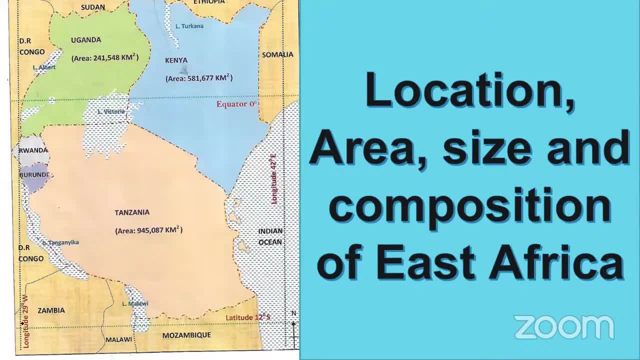 we are looking at longitudes. this longitude 29 degrees west and this is longitude 29 degrees west, and this is latitude 29 degrees west, longitude 12 degrees south and longitude 5 degrees north. then you have latitude 29 degrees west, the equator line, zero degrees. now i want us to mention the neighbors. 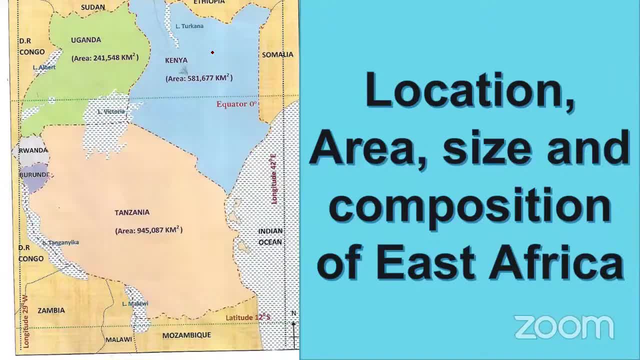 amara is saying the definition the previous person gave us was strong. the definition of what mercy? let me check you out and you clarified that amara maxi can meet you, so can say something. you're saying the definition someone gave was wrong. which definition, amara? it's our destination of latitude and longitude. how we said, latitudes are imaginary lines. 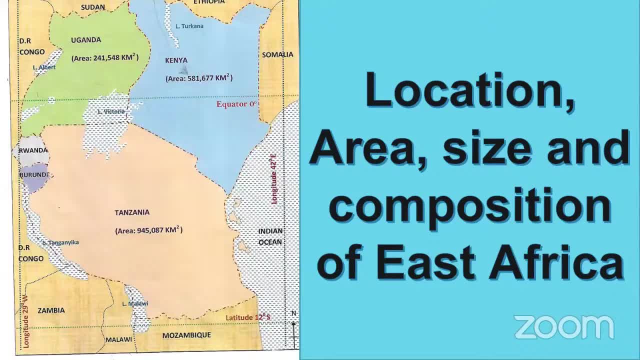 it's like. no, they are not imaginary lines, those are lines of life. oh so what is the difference between latitude and lines of latitude? it is the same, ma si. yes, so they are imaginary lines drawn on a map showing classes running from east to west. that is, those are their latitudes, mercy, are you getting it clear? 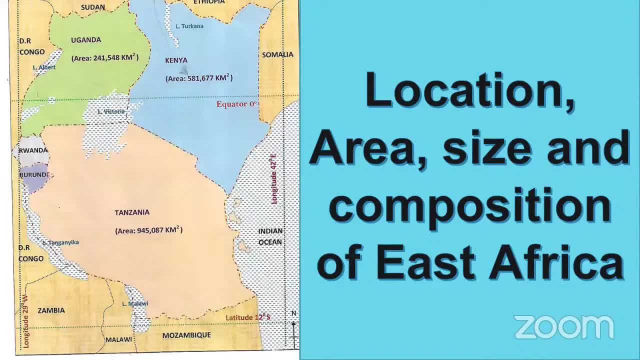 then longitude run from south to rather from north to north are only common hablando latitudes, Rather from north to south. Okay, I've gotten your concerns, Masi. I'm glad I've clarified it. Let's continue Now. when you look at this, what are you seeing on this map? 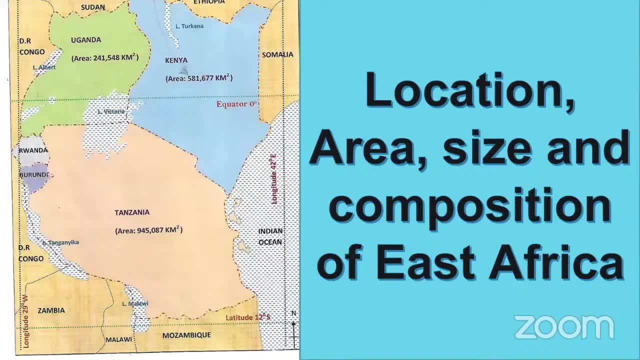 What are we seeing on this map? Tell me what you're seeing. Unmute yourself and say something Uh-huh. What are you seeing on this map? The map is showing us the location, area size of East Africa. What are we seeing? 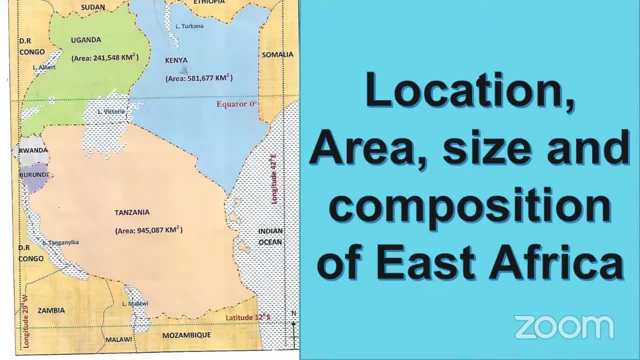 Ainamgisha, I can see the area. I can see the area of the countries and neighbors, Uh-huh, yes, Good enough. She's saying she's seeing area. I think there's the option of areas. She has seen area. 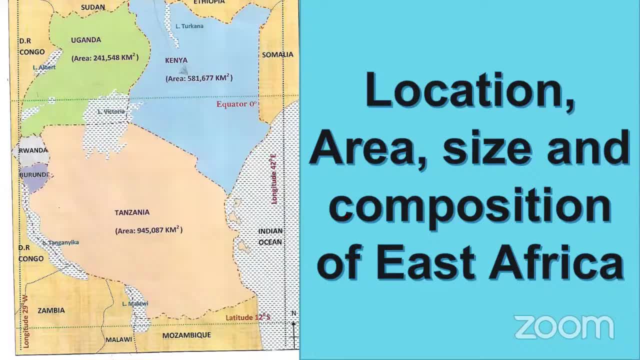 Okay, And she's also seeing the neighbors. That is what Ainamgisha, She's saying. Rodney, what are you seeing, Rodney? what do you see? I hope you're taking notes, Rodney. what can you see, Teacher? I can see the Indian Ocean. 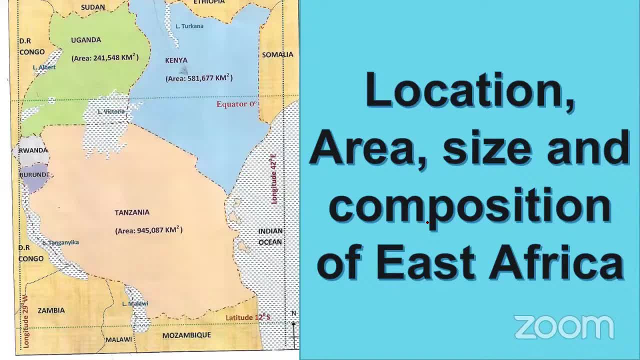 Rodney, you're seeing the Indian Ocean, Mozambique, Malawi, You're seeing Mozambique, Malawi and Zambia And Zambia, Okay, DRC, DRC, Sudan, Ethiopia and Somalia And Sudan, Ethiopia and Somalia. 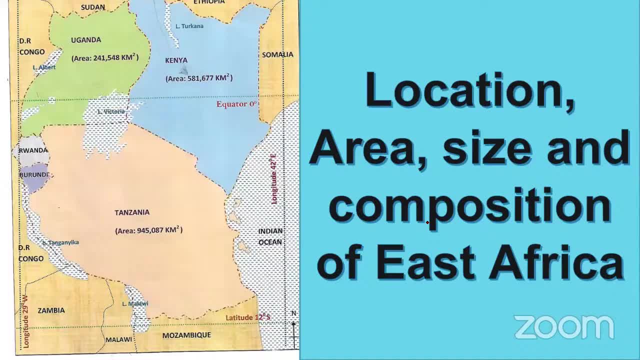 So what is common about those ones that you have seen? He has seen the Indian Ocean. Rodney has seen the Indian Ocean. He has seen Mozambique. He has seen Malawi. He has seen Zambia, DRC, Sudan and Somalia. 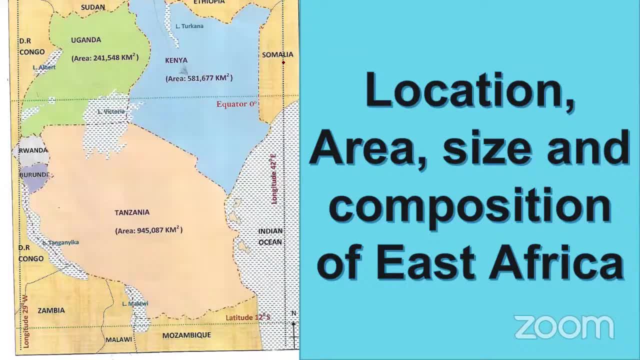 What bracket can we put these ones Under? what bracket can we put what Rodney is seeing? Melody, help Rodney, Put what he has seen in one bracket. What are they, Teacher? I think they are not landlocked countries. They are not landlocked countries. 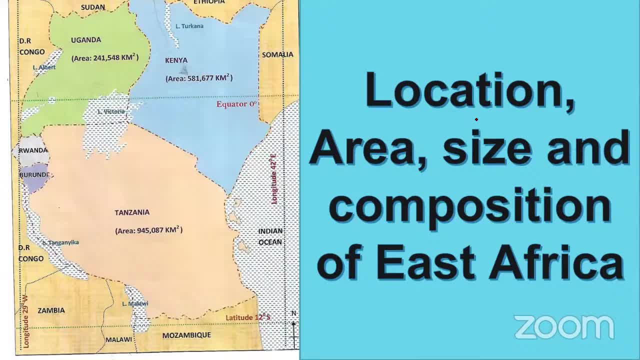 Okay, That's a Oh, my Neighboring countries of East Africa. Beautiful Rodney has seen the neighboring countries of East Africa, So give me the direction, Gloria, Priscilla, give me the direction that I'm going to mention of this country as far as being a neighbor. 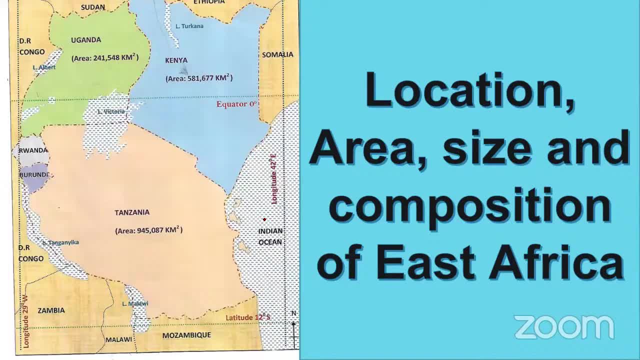 East Africa is concerned. okay, The Indian Ocean, Which direction is it? The Indian Ocean neighbors East Africa in which direction? Or borders East Africa? in which direction? Which direction is this? Melody Faith? which direction do we find the Indian Ocean in East Africa? 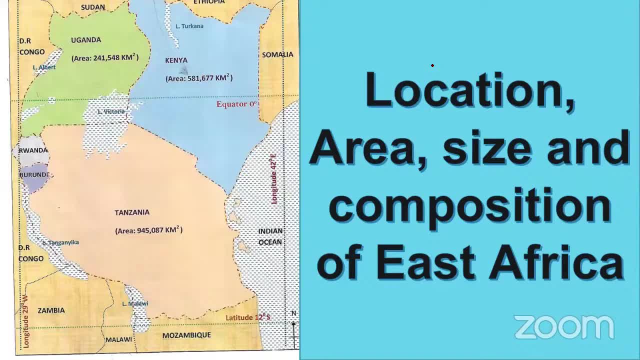 Yes, please, Oneji. Chimera say something. Chimera say something. What is the direction of East Africa, of the Indian Ocean? May I, May you, May I get a question? Yes, please, Mm-hmm. 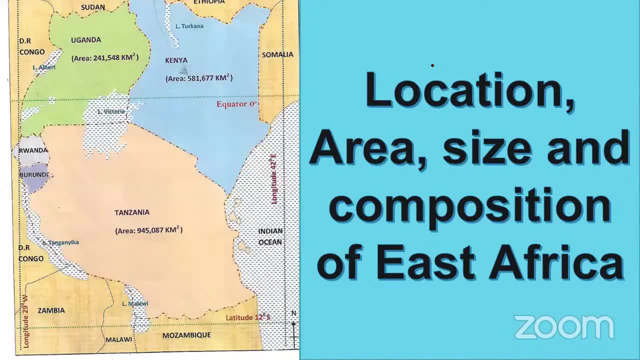 Which question Do you want to pose for us? Okay, hey, you've not had the question. i'm saying: what is the direction of the indian ocean as far as being a neighbor of east africa is concerned? which direction do you find the indian ocean if you're standing in east africa? what is the direction of the indian ocean, chimera? 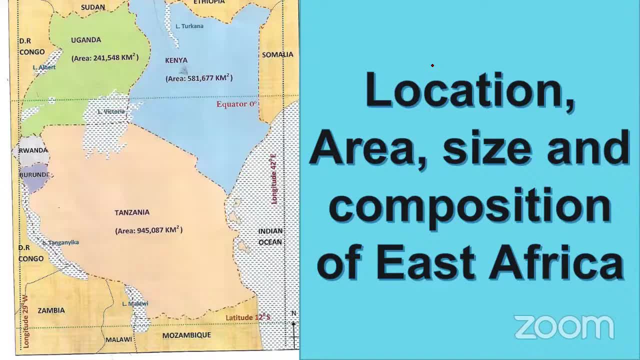 let me help him. you don't know, it's the east. it's in that the east, beautiful. so in the eastern part of east africa, east africa is bordered by the indian ocean, which other country borders east? in the east, emma, which other country borders east africa? in the east, 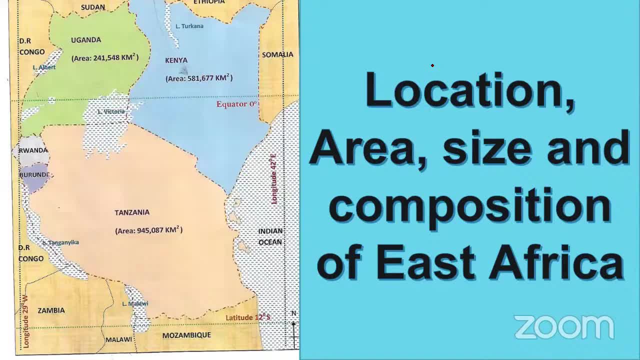 emma? which other country borders east africa in the east? Sorry, Emma. which country borders East Africa in the east? Sorry, Thessaly's, Thessaly's. Okay, I want us to look at what is on the map. 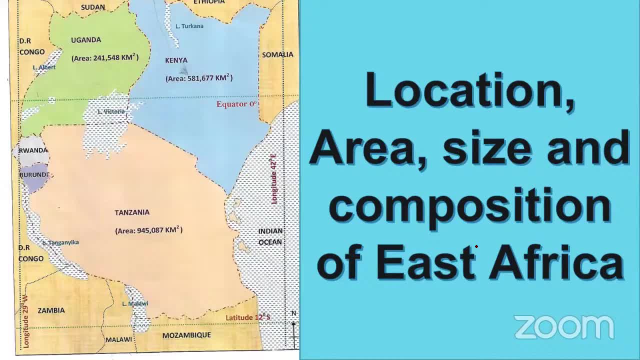 Follow what is on our map and give me the proper answer. Drusilla, my name's. which country borders East Africa? in the east? We've mentioned one was the Indian Ocean. What is the other one? Water country? Yes, the country. 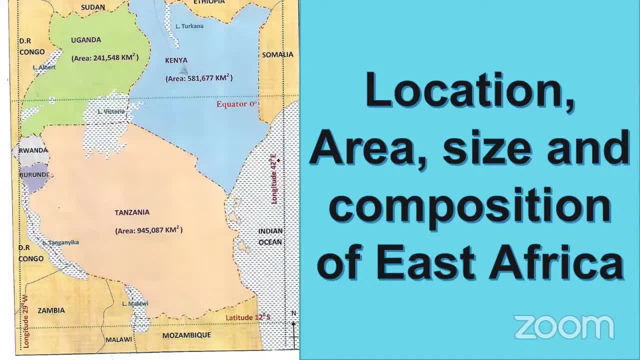 It can be Madagascar. It can be Madagascar. Okay, Good, Let's move on. Which country borders East Africa in the north? What Do we see in the north? Which country borders East Africa? We are looking at the neighbours of East Africa. 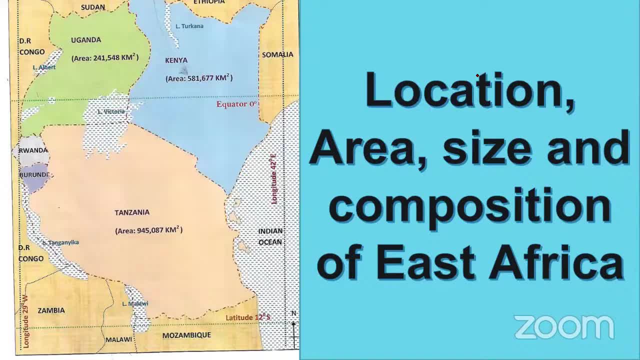 I told you, when you're studying East Africa, you basically look at Uganda, Kenya, Tanzania, Rwanda and Rwanda- Good. So which country are we looking at that borders East Africa in the north? South Sudan- South Sudan- Good, Ethiopia. 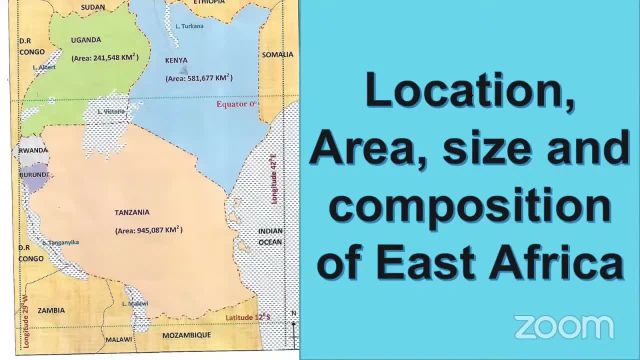 Ethiopia in the north? Beautiful. Then in the south. which countries do we have in the south? Mozambique, Malawi, Malawi and Zambia? What about the entire west? The west is covered by the Democratic Republic of Congo. 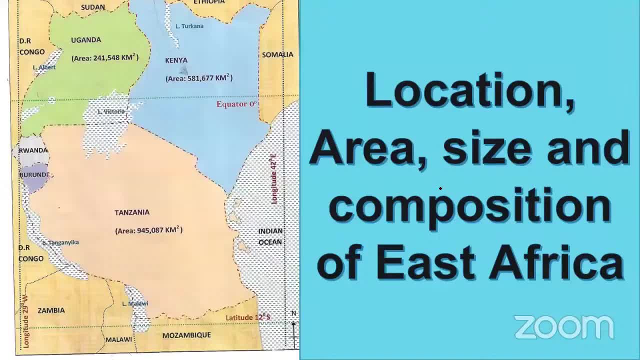 Good. Thank you, Rodney and Drusilla. Now I want us to continue. Welcome And fill this table. Fill this table. Excuse me, teacher. Yes, please, Teacher. does it mean that when a country is in the East African community? 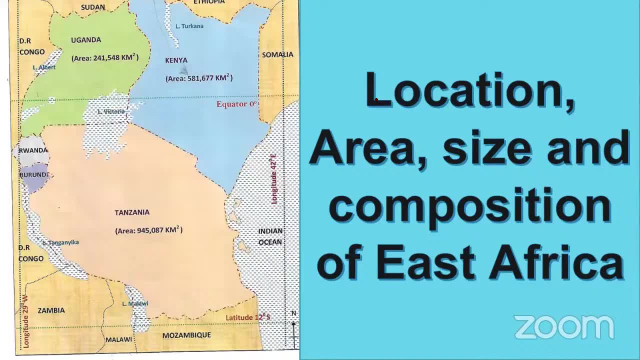 it becomes like South Sudan. Does it mean it's also in East Africa? Yes, it is in the eastern part of Africa. Don't confuse that too. yeah, When you look at the entire continent of Africa, if you can remember the entire continent of Africa. 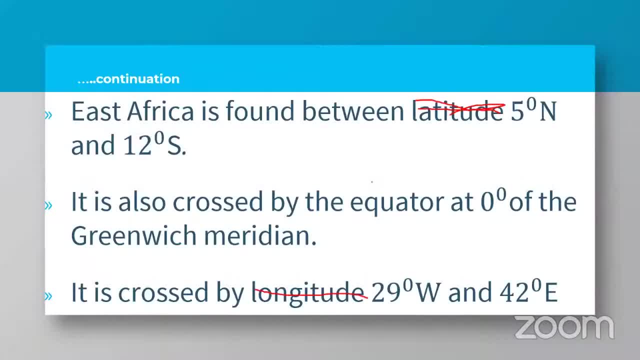 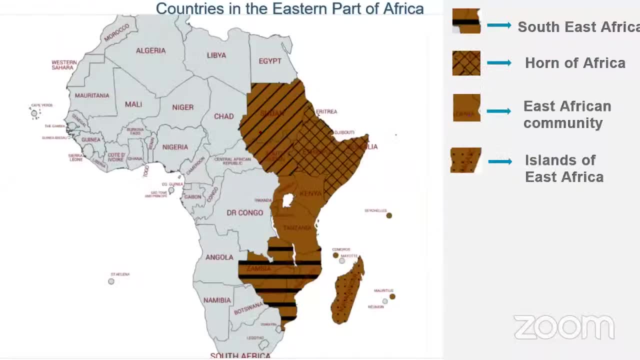 we looked at countries that are in the East African. This is the entire continent of Africa. So the countries in the eastern part of Africa, the entirely eastern parts that come from there, all of them are in the eastern part of Africa. But for our geography, as far as our geography is concerned, 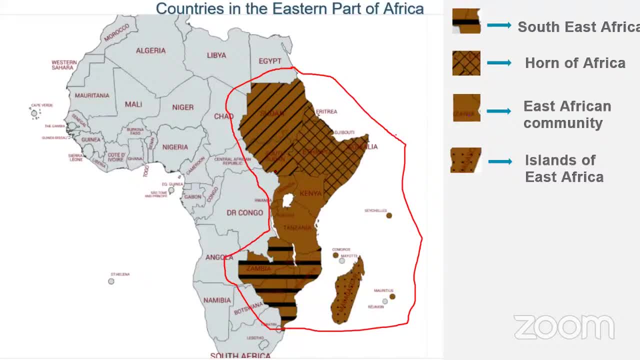 we basically look at East Africa. This is where we study As far as our syllabus is concerned. are we together? Yes, That is what we look at. Yes, But if you talk about East Africa, we mean all the countries. 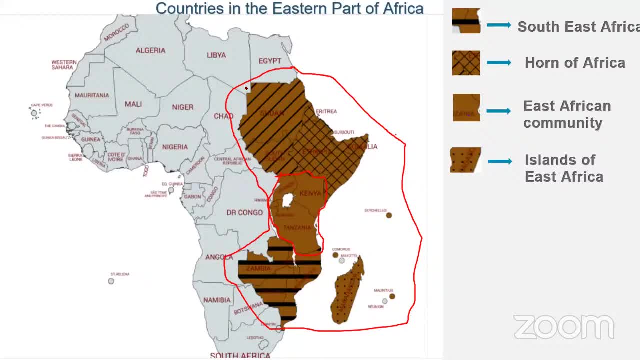 in the eastern part of Africa. Are we understood? Yes, So even South Sudan is in the East African. it joins the East African community, Just like Rwanda and Burundi, as well as Kenya, Uganda and Tanzania. So for our study, 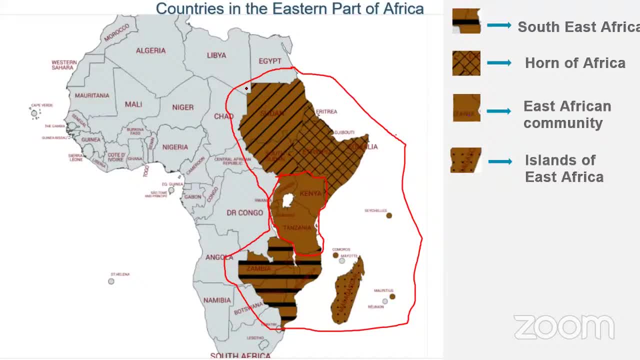 when you look at the topic relief regions of East Africa, we are basically going to analyze Uganda, Kenya and Tanzania. That is as far as our syllabus is concerned. But when I talk of Eastern Africa, the countries in the entire, when I look at the entire continent of Africa, 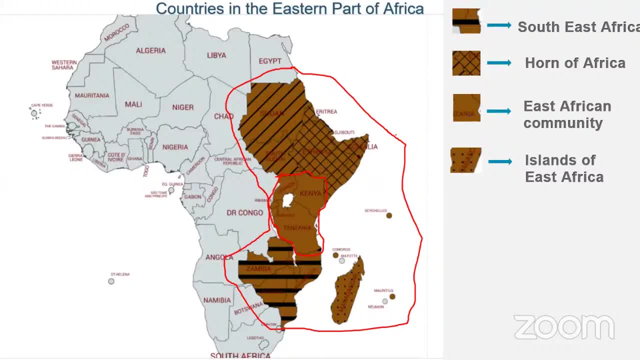 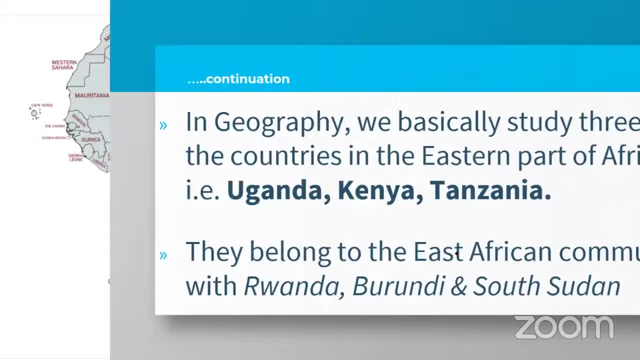 and I go into the countries in East Africa. that is what I am talking about. I hope I have answered you. Yes, Good, I am glad. So we move on. We are looking at this East Africa Now, when you look at this map. 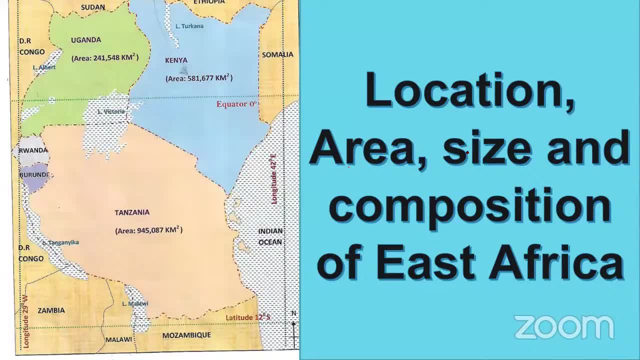 which is the largest part in East Africa, Which is the largest country in East Africa- Tanzania, Someone werender- and Burundi, ain Ist Africa or Central Africa. Yes, They are found in the center, but they're also considered to be East African countries. 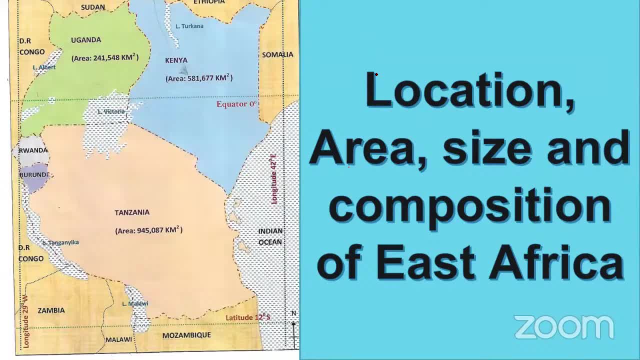 Jase, I hope I've answered you. Yes, we group them under East African, though. by location- you see them in the center, Okay, But by demarcation we put them under East African Where, under East African countries, which is the largest. 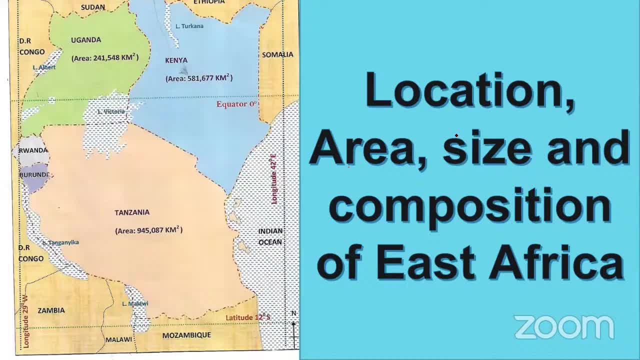 I was asking before Joyce interjected. It is Tanzania. Why? Because it has the area of 945.. This is the area of Tanzania. Compare this. And which is the second largest area, Kenya. It has 581 square kilometers, So the land in Kenya is that big. 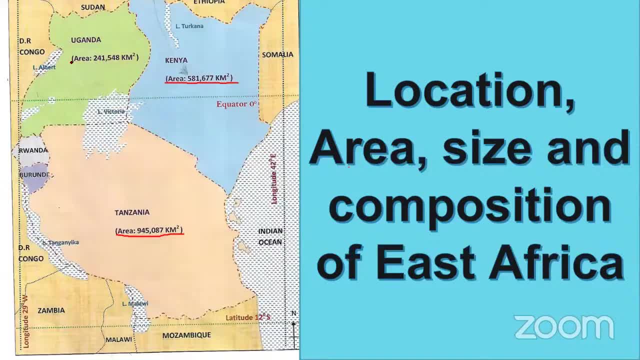 While in Uganda, I think Uganda will double Kenya, Or Kenya doubles Uganda, which is which? So Uganda is the smallest, isn't it? so In our syllabus, Uganda is the smallest. Okay, I'm going to pose another question about capitalism. 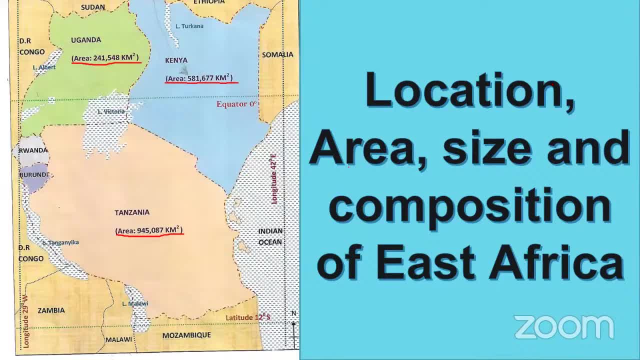 So we have looked at the location. we now know the neighbors, we know the latitudes that cross, we know the neighbors, the water bodies there. We have really understood what East Africa is about, especially regarding our syllabus. Now I want us to complete this table. 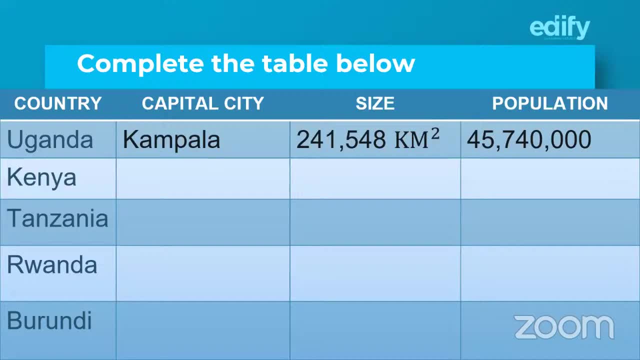 Okay, I want us to complete the table. I want us to complete. You give me the table. you give me the country, the area, the size and the population and the current statistics, by the way. Okay, We are filling this table as a group. 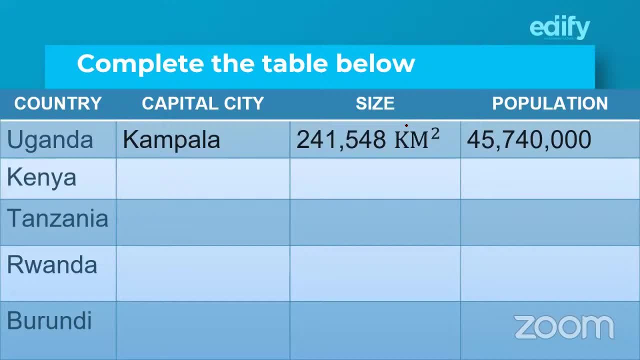 Pick something. you're going to answer Someone with an iPhone. tell me why don't you rename: Yes, Kenya, Kenya, Uh-huh, She's filling Kenya. What's the capital city of Kenya? Nairobi, Nairobi, Good. 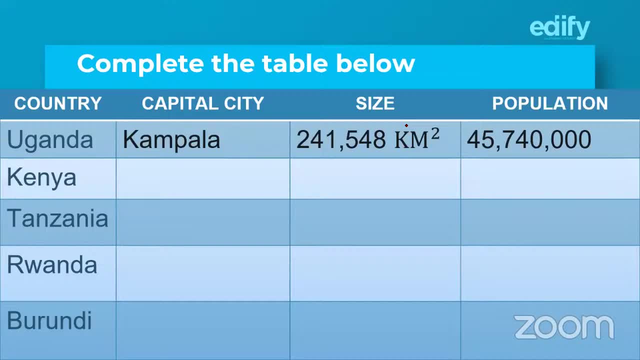 Uh-huh, I want someone to fill the other part. Who knows the population, the area size? We have been discussing the area size. Who is filling in? So if we have here as Nairobi, So that one, we have Tix. 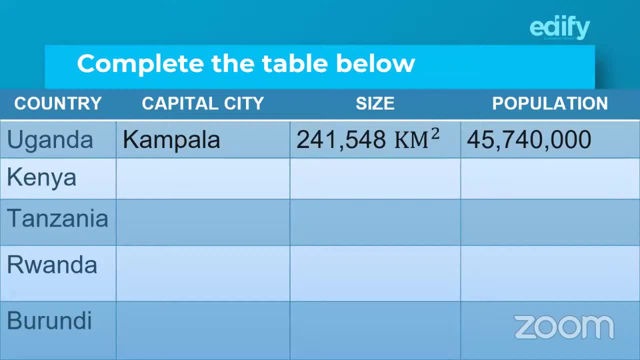 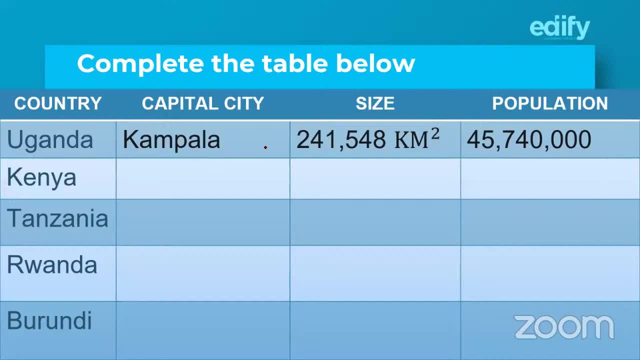 Excuse me? Yes, I can hear you. Are we going to give the? are we going to give the size of the, The country team, of the whole country, The whole country, Drusilla, That area of the whole country? 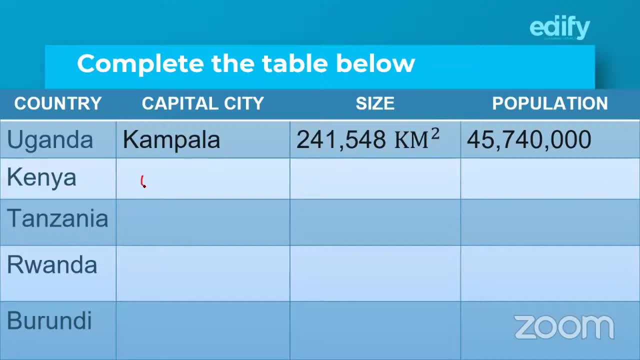 Uh-huh, have finished kenya. someone has said the capital city of kenya is: we have finished that one. i want someone to fill this one the size of kenya. who still remembers the size of kenya? the map has just been in your face. pretty, pretty. say something. what's the size of kenya? 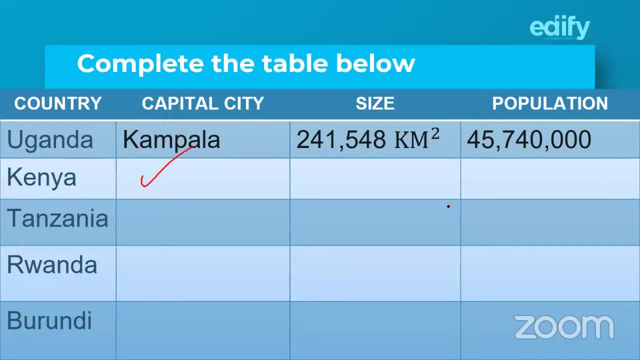 money. good morning, what is the size of kenya pretty? what is the size of kenya pretty is not with us, drusilla, drusilla. i want to hear from someone else, my dear philliam, what is the size of kenya? find something. you feel this table okay, pretty now you and 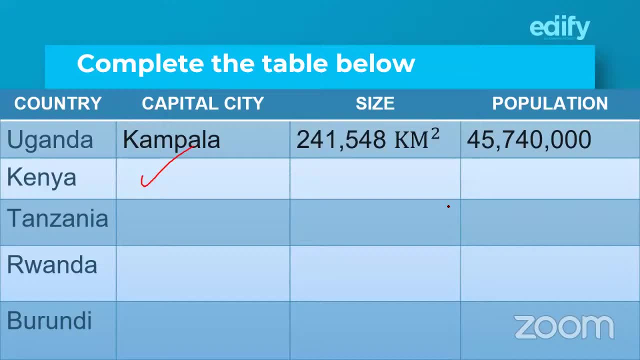 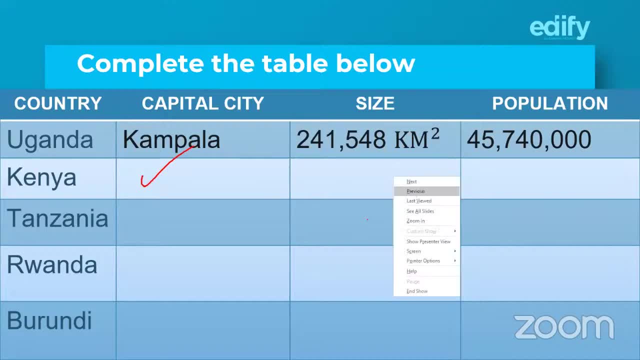 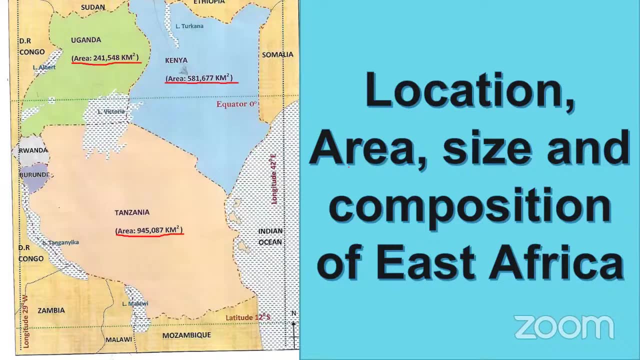 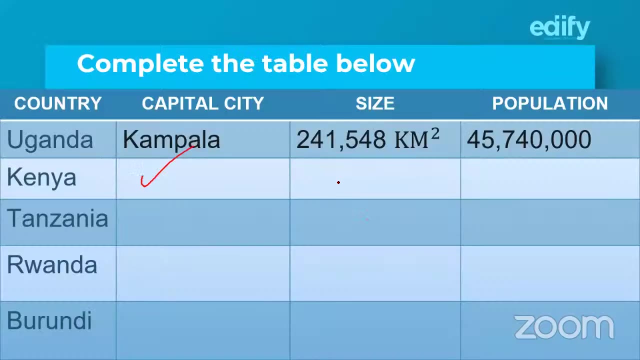 i'm not sure. i'm not sure, i'm not lying to us. oh, let's look at this. so it is 581 thousand 677 kilometers. thank you, prudence, uh-huh. so even for kenya. we have looked at that. we have filled the platform, guys. 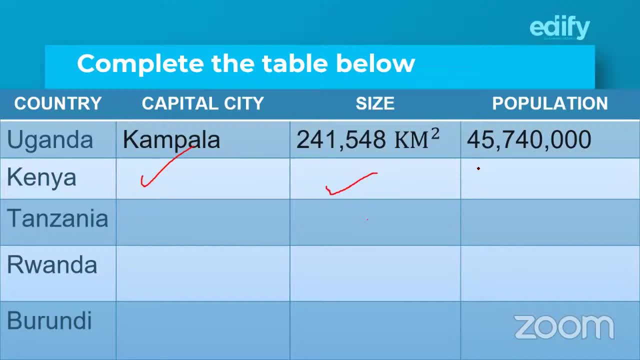 what is the uh population of kenya population? who knows the current population of kenya out? yeah, i'm hoping you do your assignment meanwhile because, yes, how many people are in kenya? 44.3, 44.3. that is according to which statistics? because i have the most recent, the 2020 world. 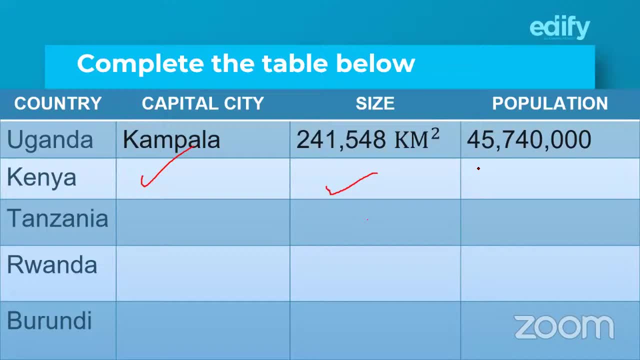 bank statistics 2019. don't you see we need done for 2020.. uh-huh, jace, what are you able to feel in the table? what are we able to? i'm checking. you need to do this as an assignment, so i need to. 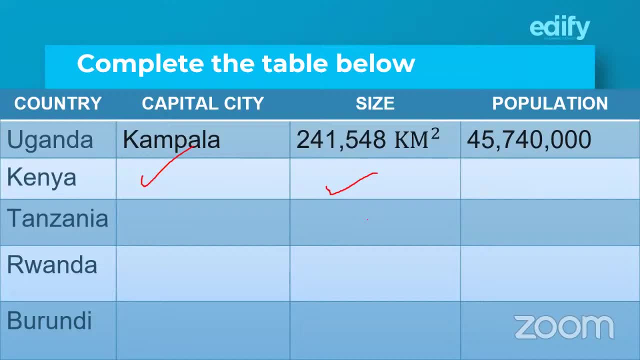 check your attention as well. kenneth, i have a kenneth. what are you choosing to feel in this table? we haven't filled the population of kenya. this is the assignment i want you to submit. emma, i see you want to say something the most. yes, emma, yes, yes, yes, emma, never want. 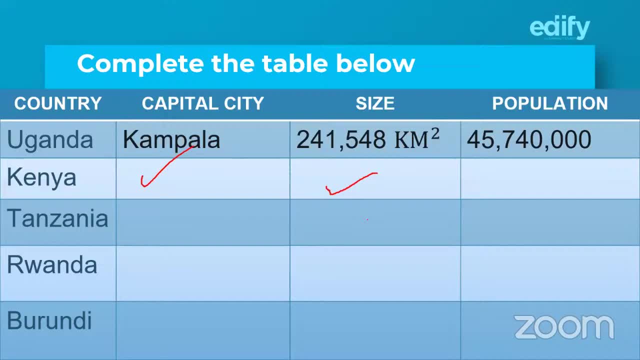 never to give the population of kenya for today. for today, uh-huh, okay, it's 55 millions. 55 million, amazing. that is the most recent 55 million. thank you, emma. i hope you are paying attention because that is the assignment i want you to fill and submit for marking. so can you imagine? 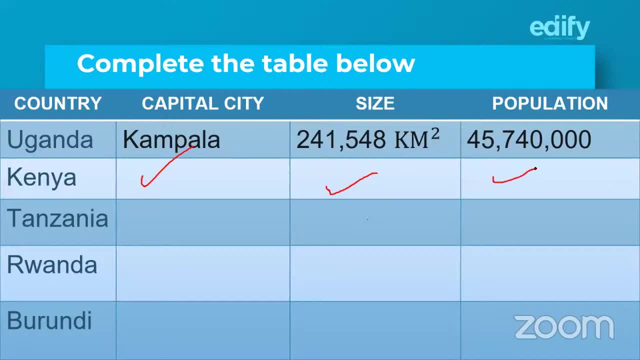 we give you an assignment and even hope you do it. so kenya is done. we move on. we move on, we are moving on. who is feeding in? who is giving us? you're giving us the wrong statistics in the chat. if your hand is up, something, yes, jonah. 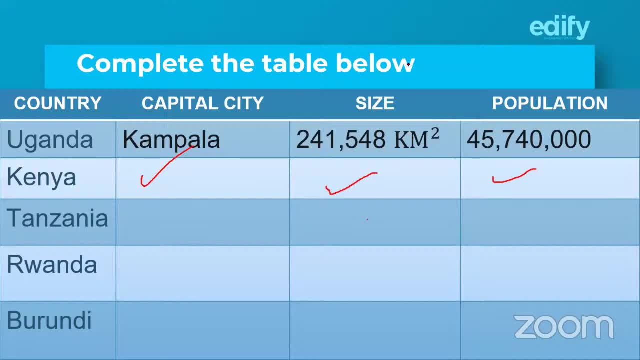 jonah of tanzania is the doma, the doma for tanzania. juna has given us the wrong statistics. we are moving on. who is feeding in? who is giving us jona? us with Tanzania as Dodoma Goods? What is the total area? 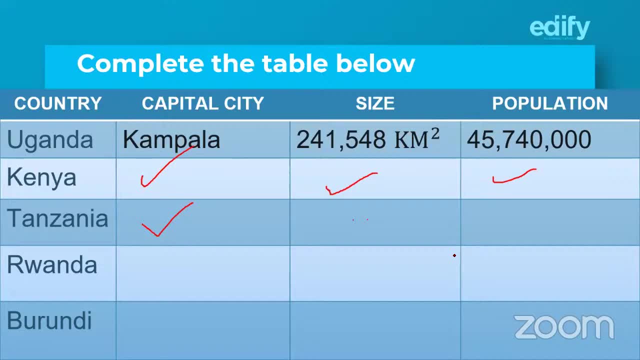 Total area of Poi Jonah. let's keep it at that. Let me hear from someone else. Nina, Nina, Nina, Nina, Are you giving me the size of Tanzania? You said Tanzania is the biggest. What is the size? 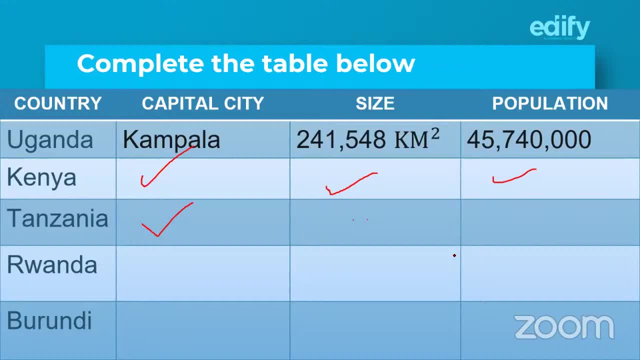 Nine, nine, nine million- I'm hearing you. Nine million for nine million, 45,000, 87 kilometers. Nine million, Nine million, 45,000, 87 kilometers. You're lying to us. Is that what we have in our map? 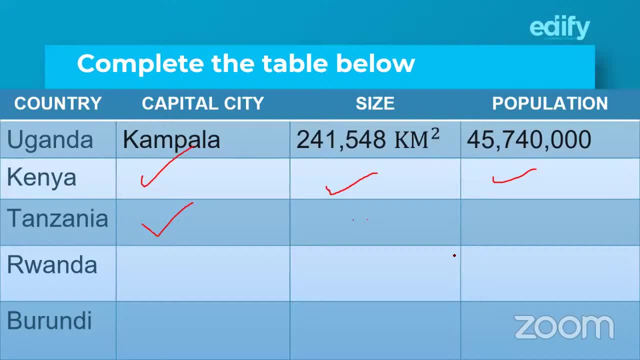 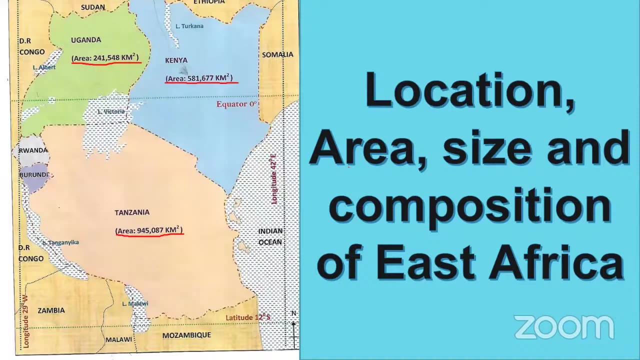 No, Jose Maria, can you help my friend Nina? Nina, I think you're lost, Can't you? Is it really nine million? Let's go back and see. Is that nine million, Nina? No, Yeah, so read it right. 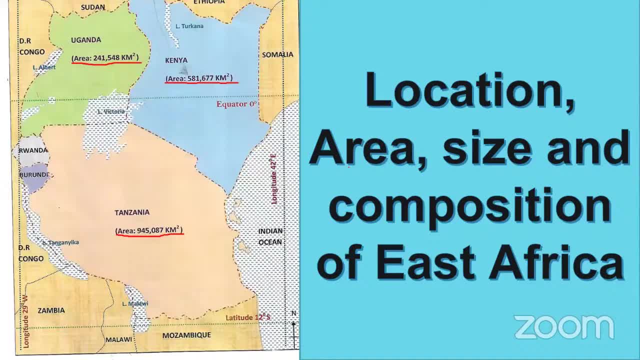 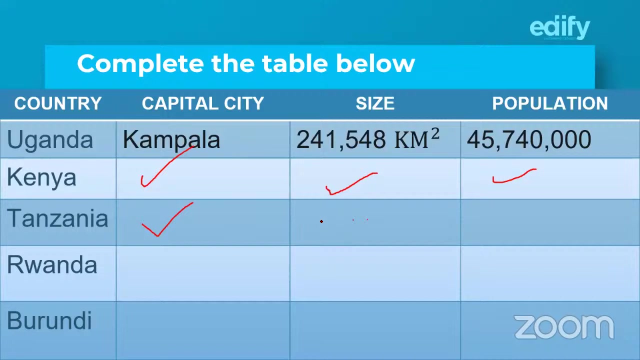 Nine nine hundred 45.. Nine hundred forty five thousand Eighty seven, Nine hundred forty five thousand Good Eighty seven kilometers squared. Beautiful, Aha. So even the size of Tanzania. We are now Kilometers squared. 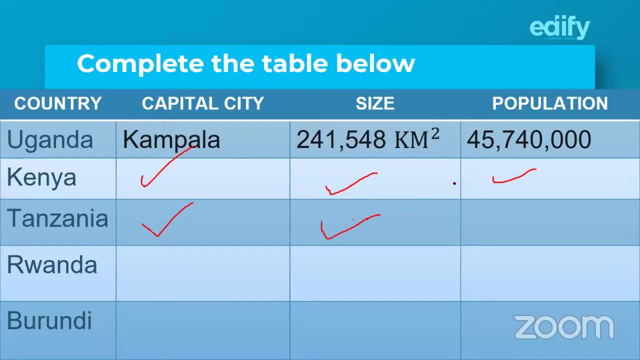 Thank you. Thank you, Nina. Who is giving us the population? Who is giving us the population? Joel and Nina? Who is giving us the population? Joel and Jesse, Say something. Joel, Okay, Nina. thank you, Mute yourself. 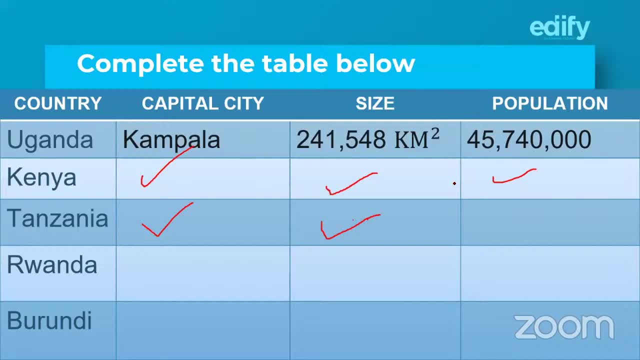 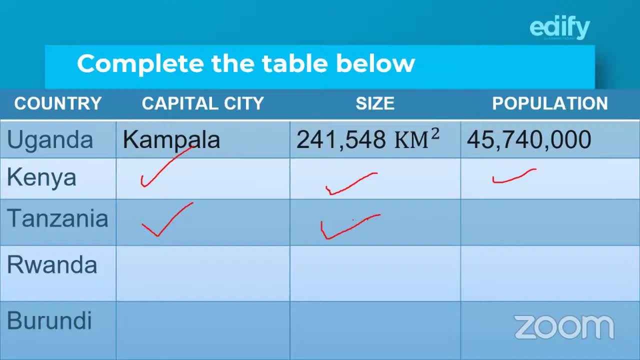 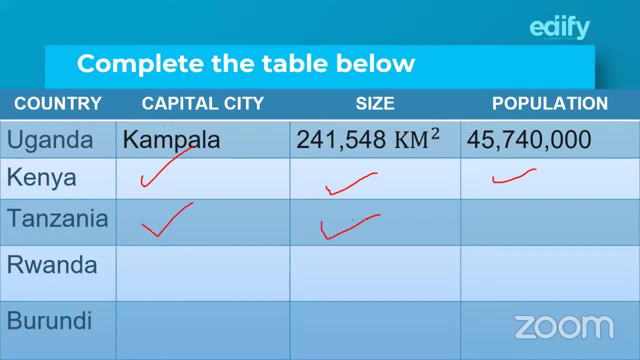 Emma, I hope you're taking note. I need this one submitted before the week ends. So you, Sixty one million two hundred ninety eight thousand sixty one million thousand. that is as far as the current statistics are concerns. so as far as giving, 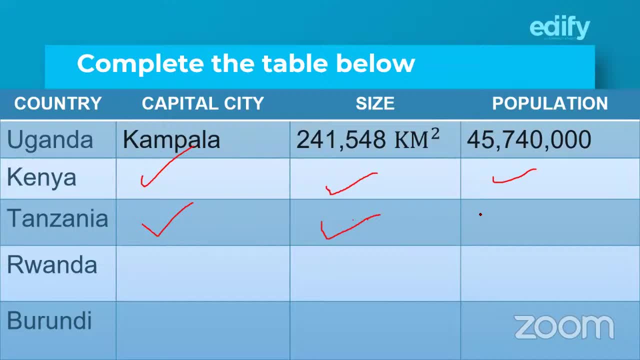 the size, the population of tanzania is concerned. i think we're also through with that. let's cross to randa. what's the capital city of randa? please, you're giving us 59 million over for which country, i don't know. asante is saying: i repeat: what should i repeat for you? 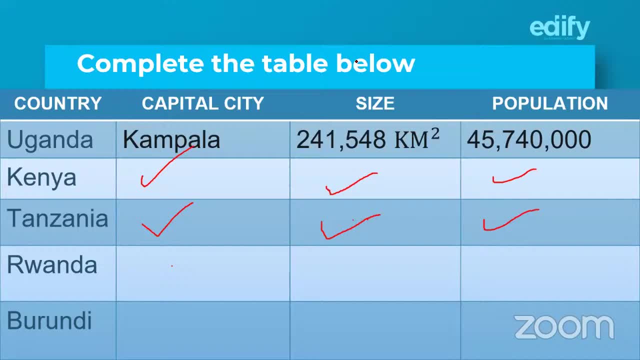 asante, i have not understood what you have not understood, because we want to move on. asante, unmute and tell me what you want us to repeat. faith has given us shigali as the capital city of tang of randa. zack, now you're frustrated. what is happening? so shigali is the capital city of randa. 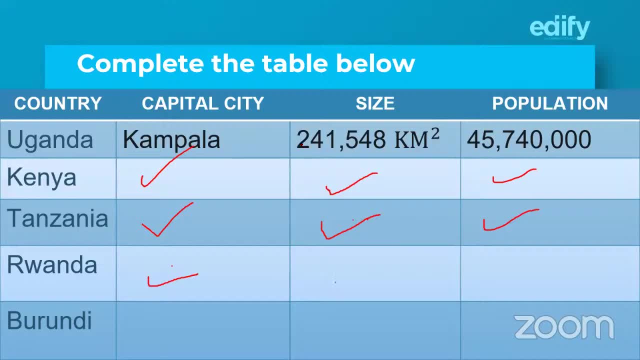 what is the size? people have risen their hands, priscilla. what's the size, priscilla? what's the size of randa? how big is randa? looks like a small country, but how big is it, priscilla? no idea, robina. what is the size of randa? 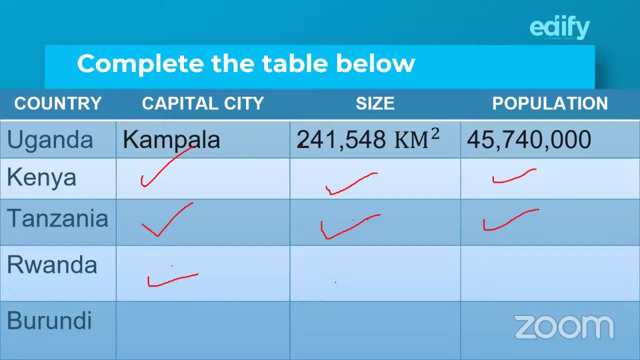 hey, you people. you mean you only talk to your neighbors. what is the size of randa? the hands are up, you're not saying who's in my life, just say something. let the gentlemen challenge the ladies. what is the size of randa, teacher? it is 26 338 square kilometers. 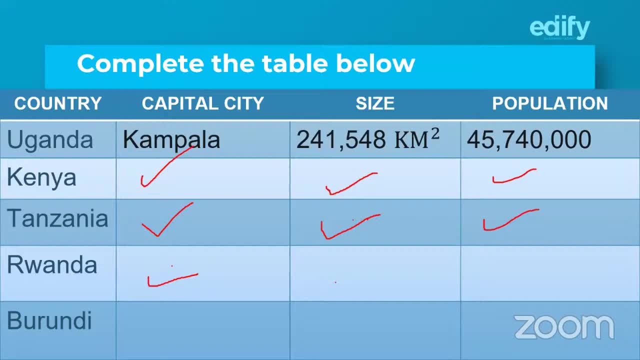 it is 26 338 kilometers, 26 338 square kilometers, are you sure? yes, where are you researching from? where are you researching from? because i feel that is not right. okay, let's look at that first. write it in the chat as you compare with us. 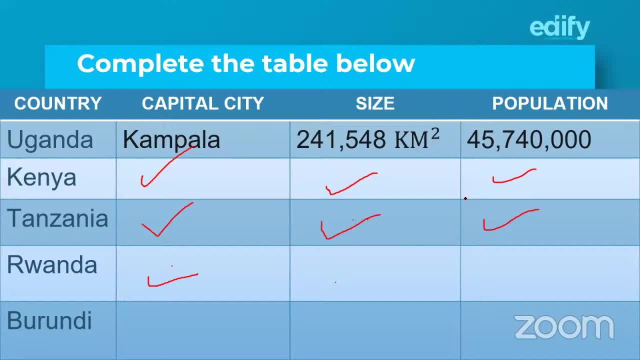 okay, let's look at that first. write it in the chat as you compare with us. who also has found out the size of randa? that is cosima's idea. elijah, let's back in. we need support. so, elijah, let's back in, we need support. so you're saying it is. 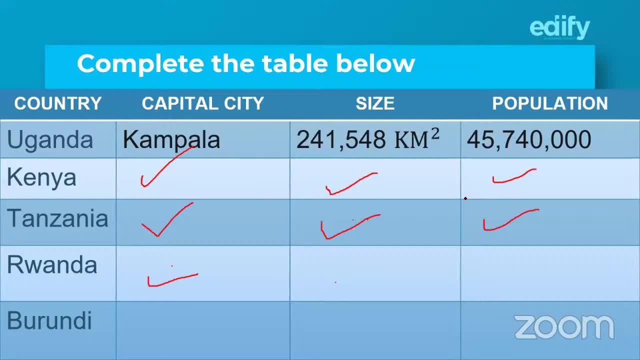 elijah, write it in the chat so that we can refer you right. the size of kenya is: i want someone to katumba, i want you to. i want someone to katumba. i want you to fight and defeat elijah. fight and defeat elijah. and defeat elijah. fight and defeat elijah what he like. do we take what elijah is what he like? do we take what elijah is what he like? do we take what elijah is saying as the truth? yes, juna. 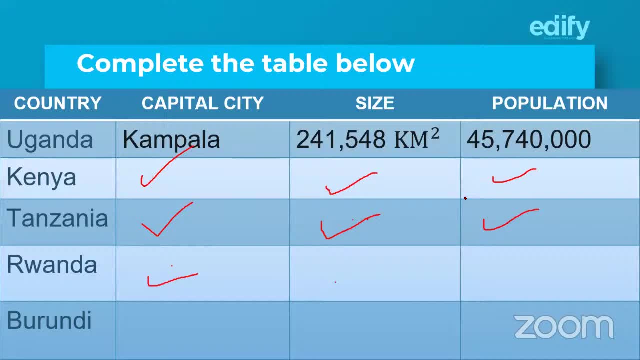 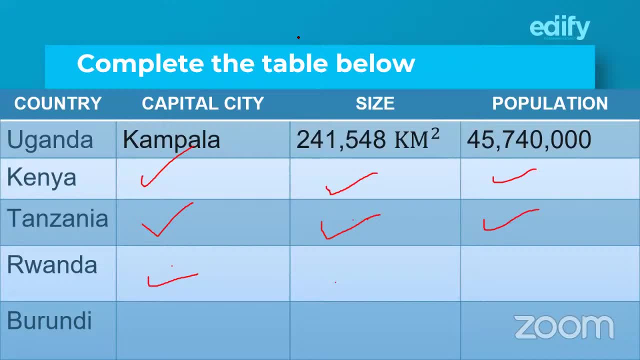 even katumba. you have the same answer: yeah, yeah, yeah, 26 338 kilometers, 26 338 kilometers, 26 338 kilometers. so i think you agree with what emma has. so i think you agree with what emma has. so i think you agree with what emma has said. 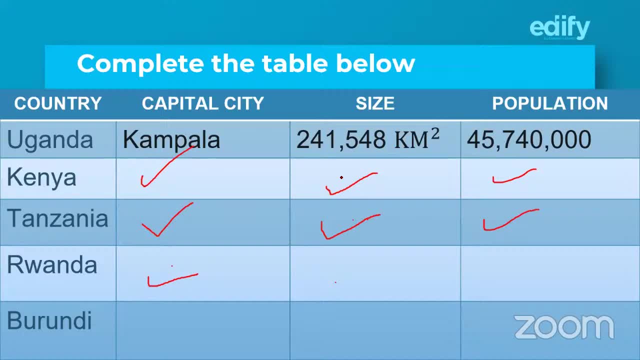 said, said even elijah beautiful, so with kenya, we even, elijah beautiful, so with kenya, we even elijah beautiful, so with kenya, we have twenty six thousand three hundred, have twenty six thousand three hundred, have twenty six thousand three hundred thirty eight. 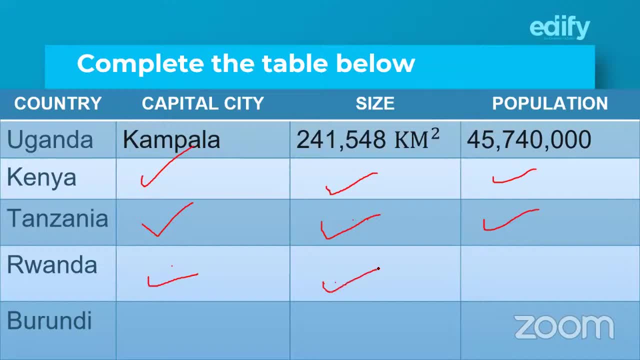 thirty eight. thirty eight people who are not paying, paying people who are not paying, paying people who are not paying, paying attention. i don't know how you answer attention. i don't know how you answer attention. i don't know how you answer this good, this good, this good, uh-huh. what is the population of kenya? 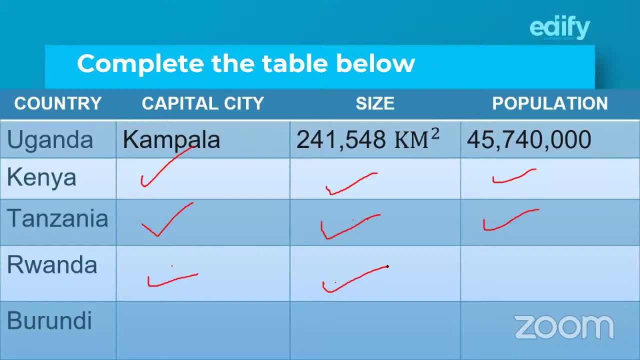 uh-huh, what is the population of kenya? uh-huh, what is the population of kenya? how big, how populated is? yes, master. how big, how populated is? yes, master. how big, how populated is, yes, master, master. welcome all on board. what is the master? welcome all on board. what is the? 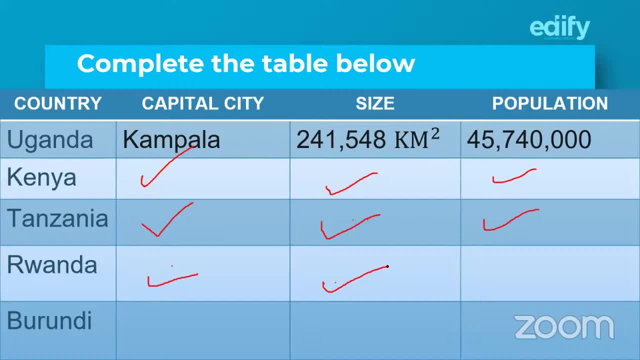 master, welcome all on board. what is the population of kenya, mother, your neighbors, what is their mother, your neighbors, what is their mother, your neighbors, what is their population? you want to go there and population. you want to go there and population. you want to go there and visit and increase their population. how? 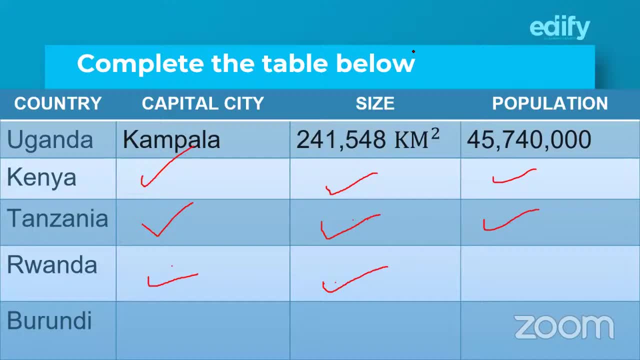 visit and increase their population. how visit and increase their population? how big is it? what is the population size? what is the population size? what is the population size? we've agreed on the size of randa. thank, we've agreed on the size of randa. thank, we've agreed on the size of randa. thank you, jenna and. 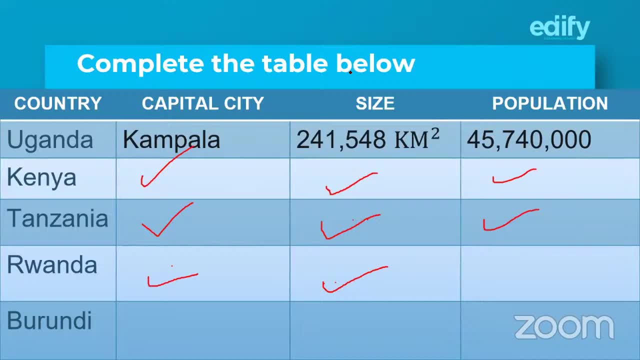 you jenna, and you jenna, and yes, yes, yes. what is the population of kenya as far as? what is the population of kenya as far as? what is the population of kenya as far as 2020 world statistics is concerned? 2020 world statistics is concerned? 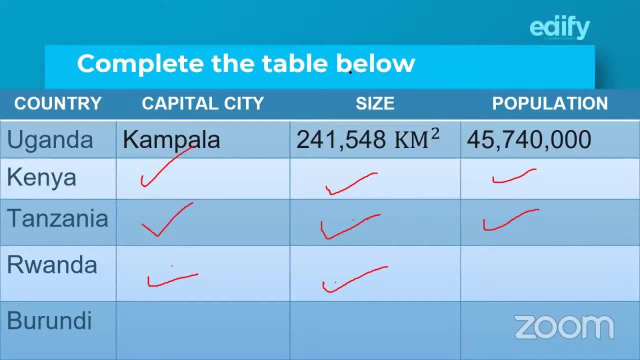 2020 world statistics is concerned. hey, matha, i was happy to see you you're. hey, matha, i was happy to see you you're. hey, matha, i was happy to see you. you're not saying anything. let me admit you, you not saying anything. let me admit you, you. 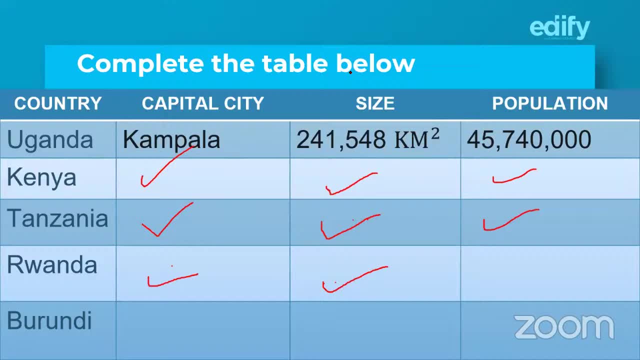 not saying anything. let me admit you. you might say this: i have not admitted me. might say this: i have not admitted me. might say this: i have not admitted me. matha, matha, matha, matha. surely you're not with us, surely you're not with us. 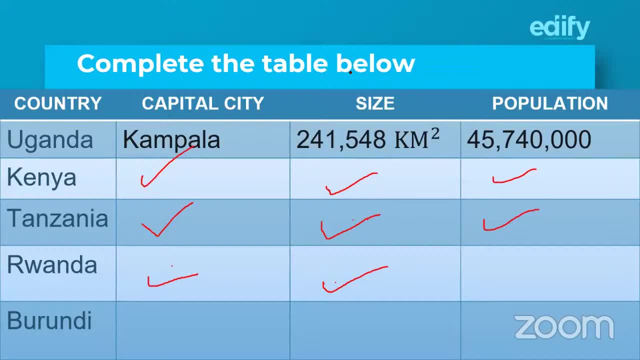 surely you're not with us? mirenbe miren: what is the population of mirenbe miren? what is the population of mirenbe miren? what is the population of kenya? remember what is the population of kenya. remember what is the population of kenya. 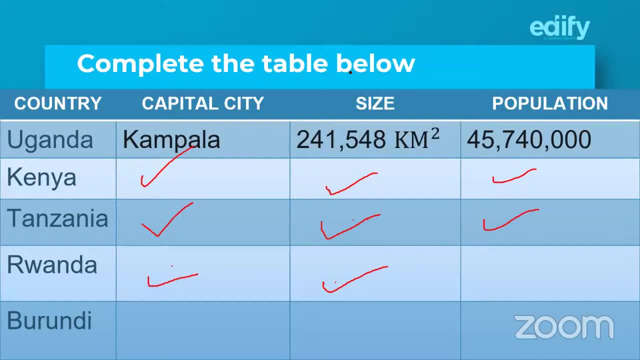 remember what is the population of kenya. blessings, some blessings, bless me with blessings. some blessings bless me with blessings. some blessings bless me with your answer, your answer, your answer: what is the population of kenya 2020? the population 2020? the population 2020? the population of randa- sorry of randa. 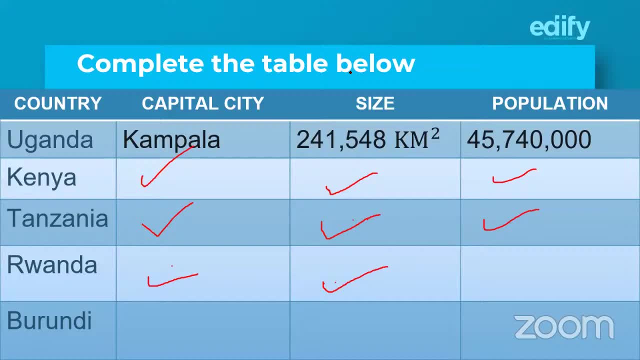 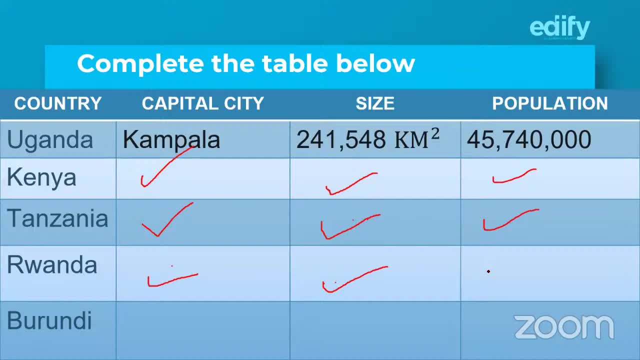 thank you 13 million three hundred. thank you 13 million three hundred 85 000 right in the chat. so as far as 85 000 right in the chat, so as far as 85 000 right in the chat, so as far as population of kenya is concerned, i think. 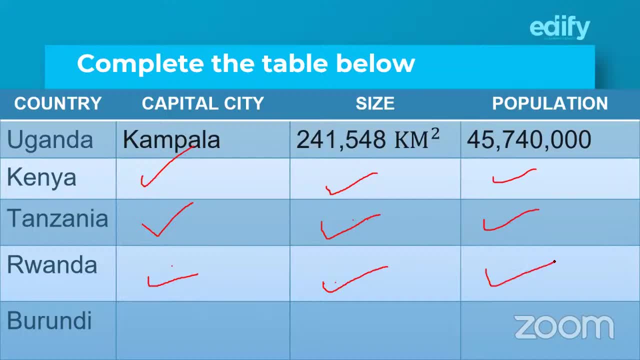 population of kenya is concerned. i think population of kenya is concerned. i think we are also done with that. we are also done with that. we are also done with that. once that work submitted. i'm checking once that work submitted. i'm checking once that work submitted. i'm checking your ability to pay attention in the 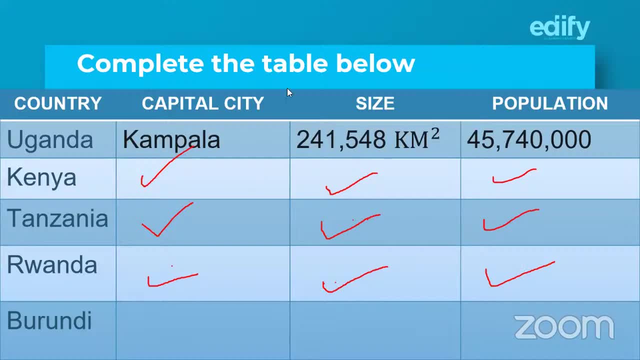 your ability to pay attention in the, your ability to pay attention in the lessons, lessons, lessons, good, good, good. let's move to the road. what is the? let's move to the road. what is the? let's move to the road. what is the capital city of? capital city of? 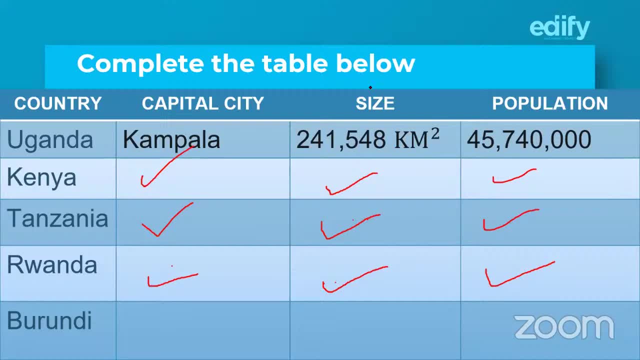 capital city of burundi, burundi, burundi. oh matthai, didn't let you unmute, but i, oh matthai, didn't let you unmute, but i, oh matthai, didn't let you unmute, but i really did. you just didn't meet yourself. 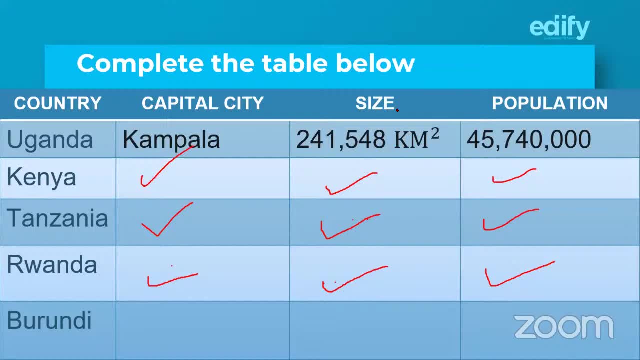 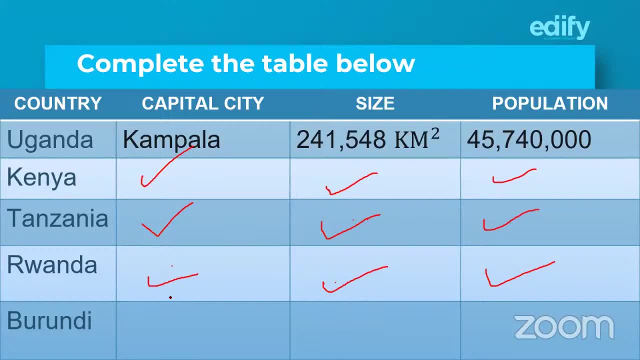 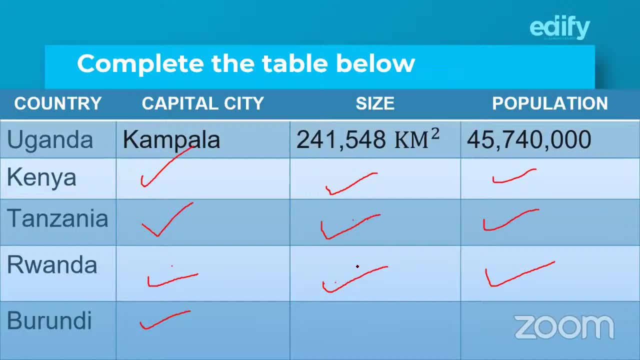 okay, size, size. size of burundi. okay, size, size. size of burundi. okay, size, size. size of burundi: itega is done size of burundi. who is itega is done size of burundi. who is itega is done size of burundi. who is giving us the size? 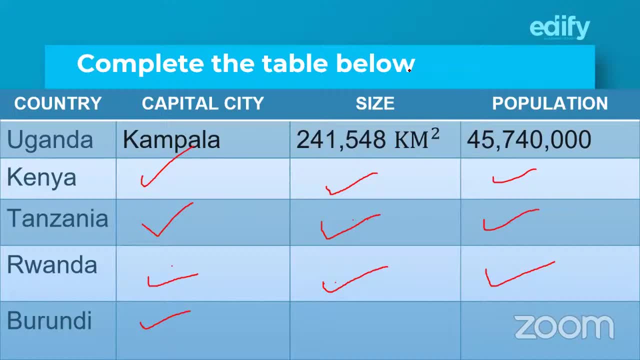 giving us the size, giving us the size. so, with burundi and randa, which is big size of burundi, size of burundi, size of burundi, hassan, you want to hassan, you want to hassan, you want to say something? yes, yes, yes, yes. 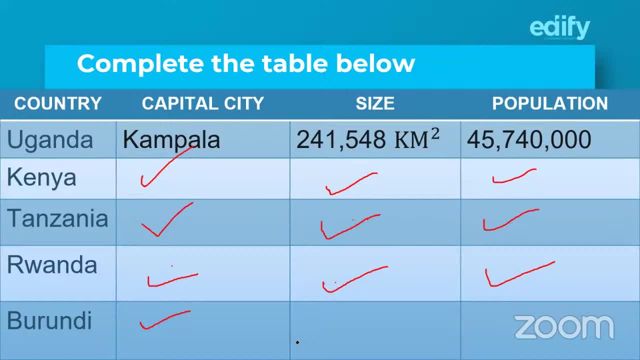 yes, kilometers. thank you, hassan. let's head to the population of burundi. now i want you to fill that table because you've all attended the class. we have filled in the answers. just fill the table and submit to your google classroom. i am already marking those that submit, okay. 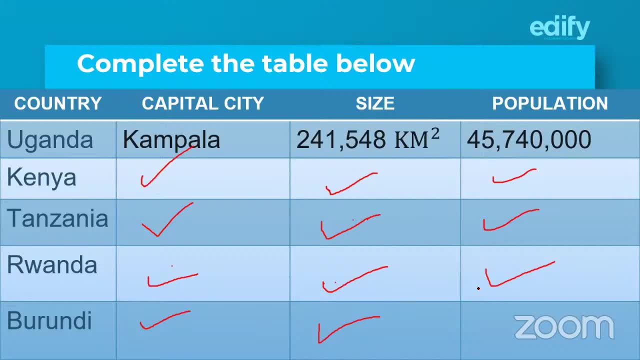 aha, gloria, what are you saying? i want to look at the population of burundi. gloria, let the lesson not end when you've been the quiet one. even god is watching you, please. what's the population of burundi? the population of rudy is 11.89 million. 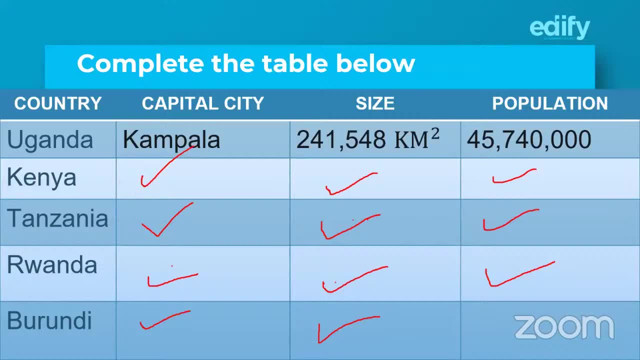 11 and you undersizing it. it is bigger than that. please thank you for trying. can i have a different version, andrew? what's the population of burundi? what's the population of burundi? let me check in the chat. someone could have given this. uh, someone begs our pardon on the size of ron d. we saved the side of burundi. 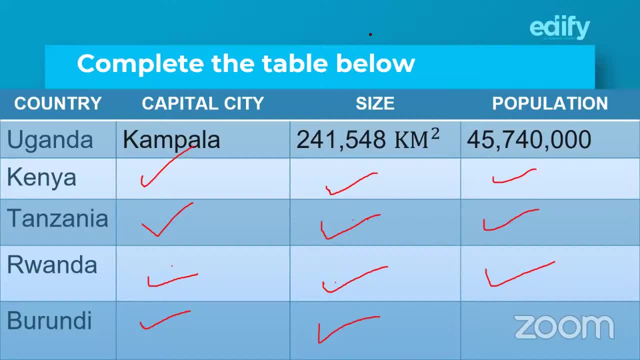 which is 11.89 million. 11.89, 0.89 million, yes, 0.89, it is 11 million 890 thousand. definitely has it right written in our chat: 11 million 890 thousand 780. oh, i think we have looked at the entire east africa now that the countries in the east african 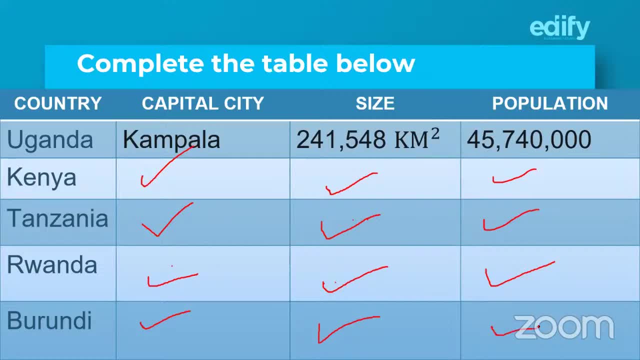 community and, as far as our syllabus is concerned, that is. that is what is going to be our major area of interest. you're going to look at kenya, tanzania and uganda. please go back home, sit down and fill that table, because you've all been in class, we have given the answers. i just want you to give that. 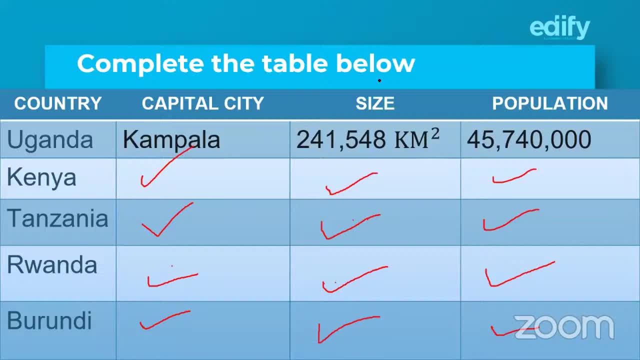 okay, fill that table and submit. someone is saying: teacher, give me the population of burundi. we said it is 11 million. it's in the chat. even daniela give us the population 11 million 890 000 and so not 12 million, 12 million 225, it is 11 million. 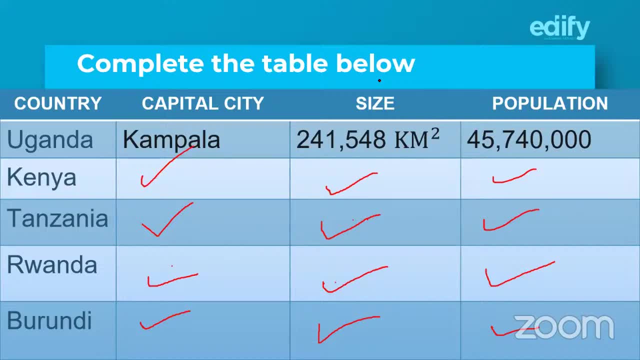 where can i hand in my work from? go to google you got. if you have a phone, go to play store and add. you get the google classroom app. then you fill in accordingly the population of tanzania. if people are not paying attention- now, chloe is there, i'm not repeating for you. that is why it. 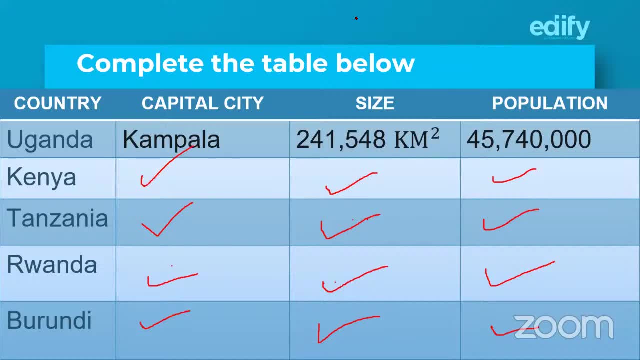 is an exercise we are filled in for you. take it upon you to fill my table and submit your work, okay, hey, i was checking your attention span during my lessons. now, when i talk of relief regions in east africa, what is relief? what comes to your mind? what is relief? 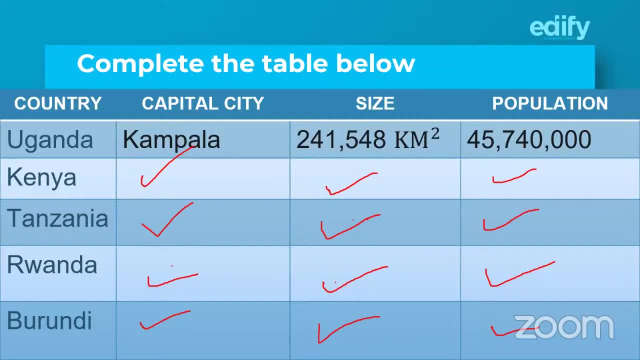 because what we have done today, we have first understood the location, the size, the neighbors of east africa, and so what is relief? we still have some time. what is relief? by description, rodney rodney? rodney rodney, you want to define for us really, when i talk of relief features or regions of east africa, what comes to your mind? 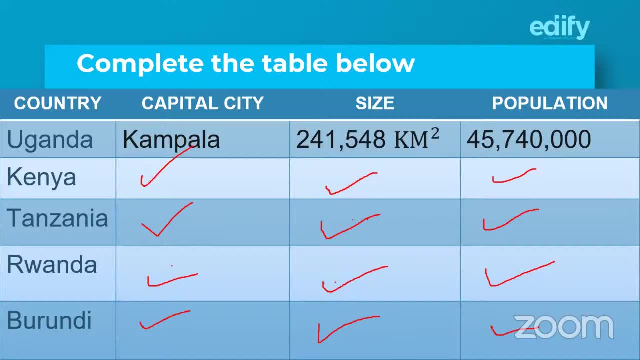 right me. yes, relief is the drainage system of an area. you look at the drainage system, rodney. okay, that's the submission. jasmine, when i talk of relief, what comes to your mind? when i speak of relief, what comes to your mind? i give this as an assignment, and i ask him who don't know yet: alvin, when i speak of relief, what comes to your mind? 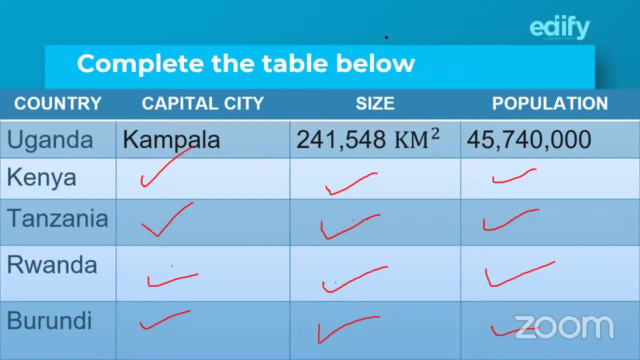 alvin noah. when i say relief, what comes to your mind, daniela, is saying relief is the natural appearance of land, of land, beautiful, thank you both. so relief, you are basically looking at the general appearance of an area. when i talk of terms of an area, when i talk of land, of land, you look at the appearance of a particular Accentが. 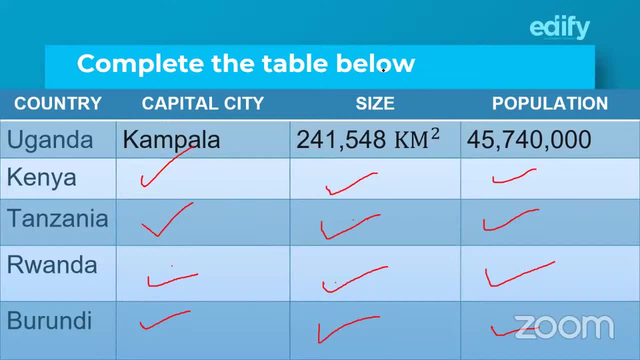 of appearance. what are the things that can compromise or comprise the appearance of an area? when i talk of the appearance, which area am i looking at? because you're saying it is the physical appearance? what are the things that in an area, what are things that give it an appearance? because those things are the ones. 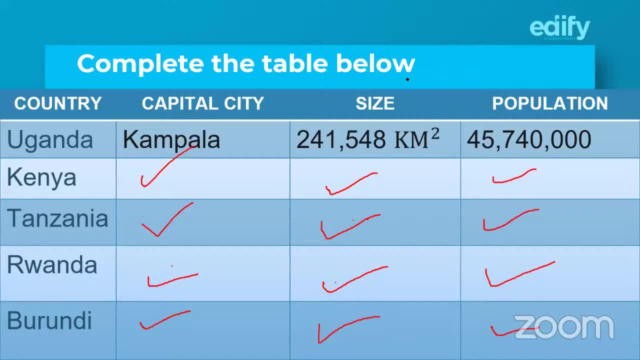 you look at as relief daniella? daniella, i've unmuted you. so when i talk about- yes, we've looked at, it is the appearance of an area. so what appear? what things do we look at? describe rodney: he's tall, he has big eyes. the appearance of rodney is that when i talk. 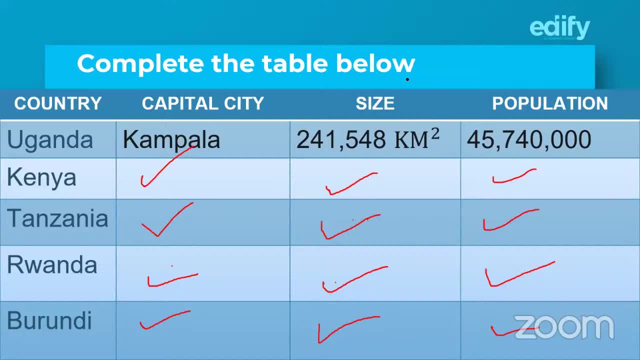 about appearance of an area. what things am i going to look at? the sloppiness of the area- uh-huh, the sloppiness. so i'm going to look at the steepness or the sloppiness of the area. good, what else am i going to look at? 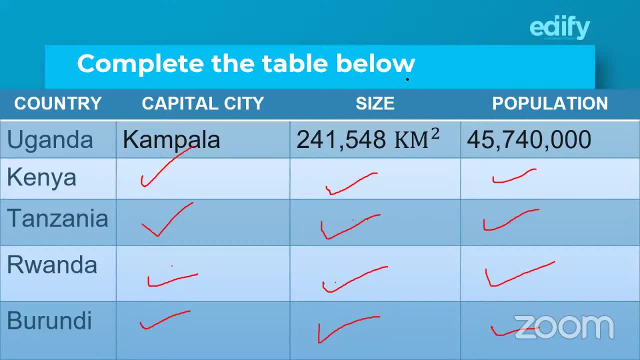 christine, thank you for raising your hand. christine, say something. yes, what when i talk of general appearance right in the middle of the area, right in the middle of the area? yes, what when i talk of general appearance right in the middle of the area? yes, what when i talk of general appearance? 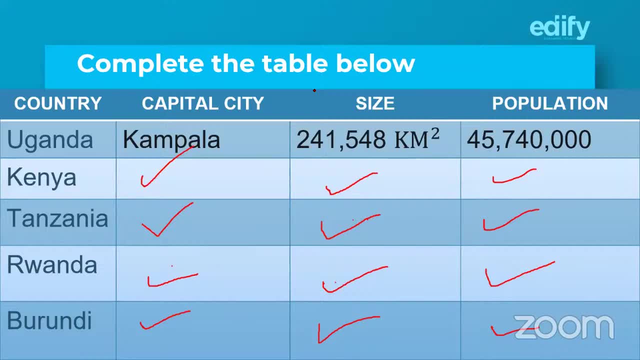 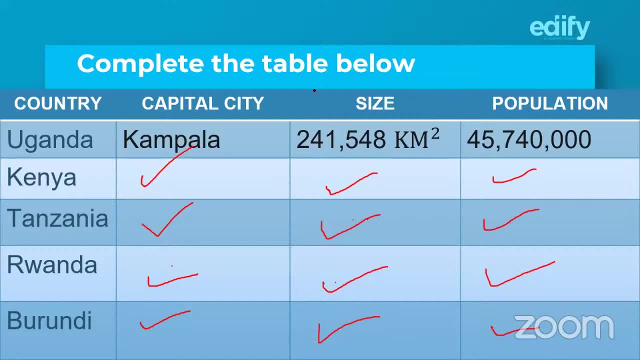 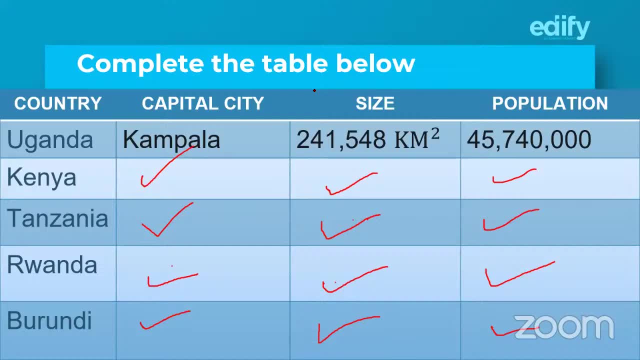 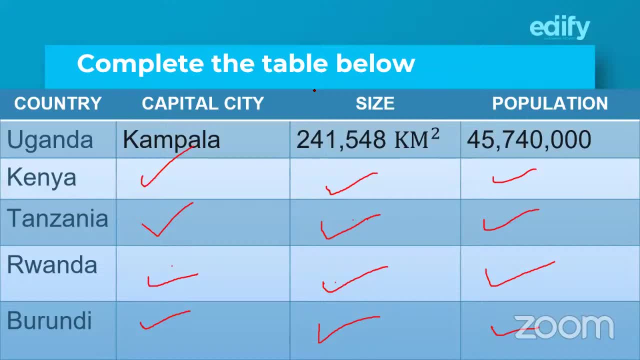 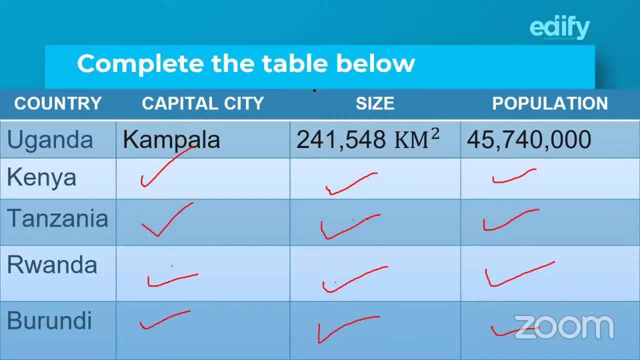 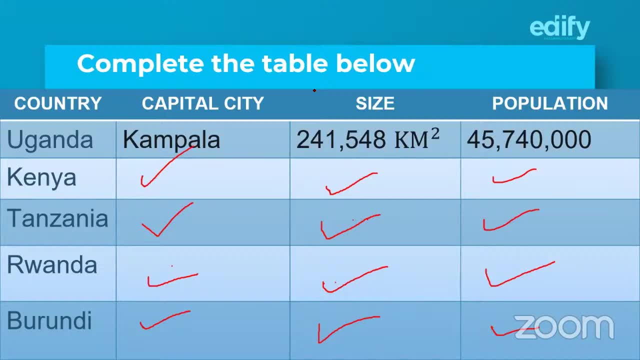 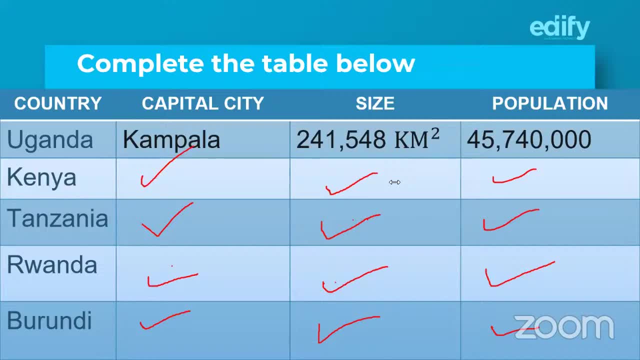 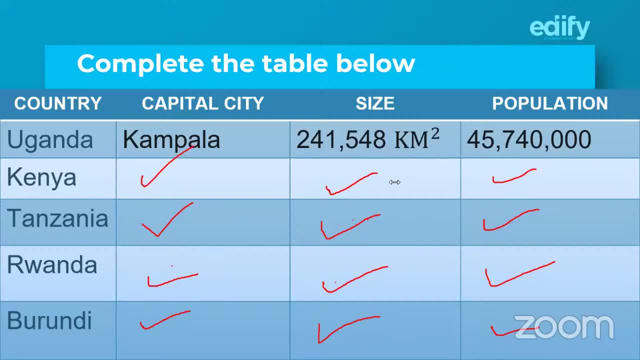 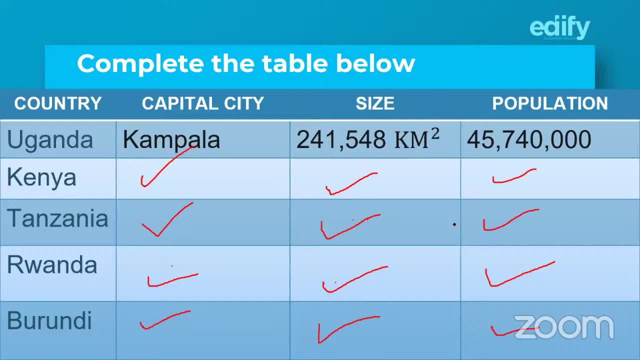 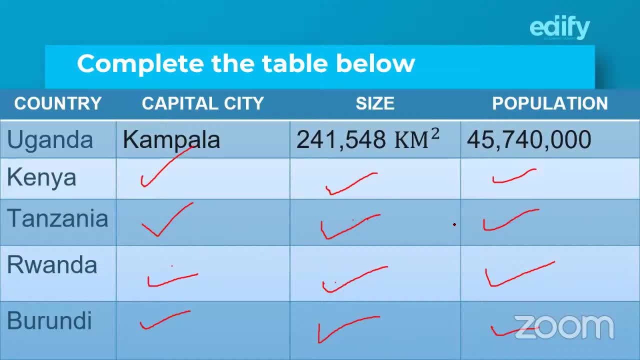 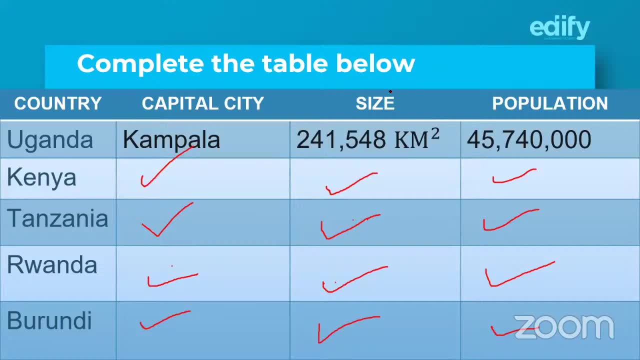 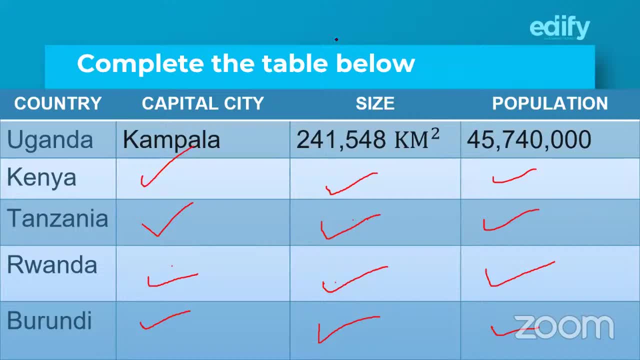 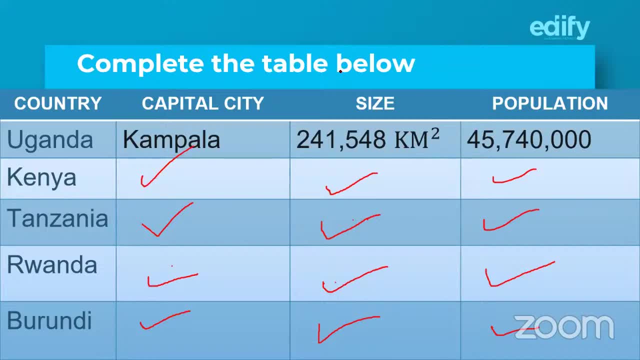 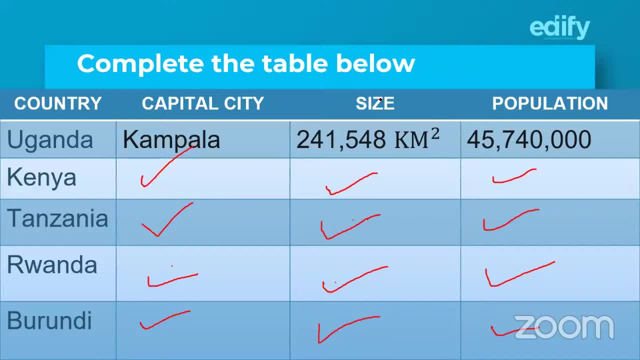 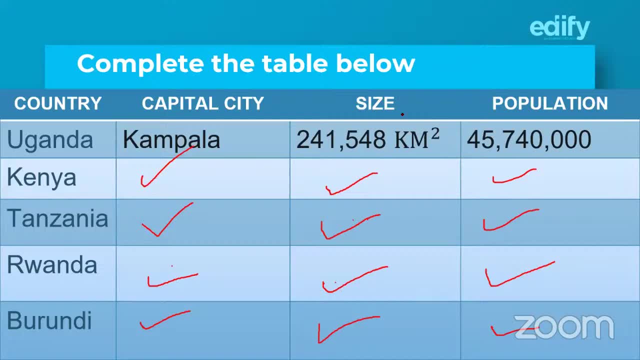 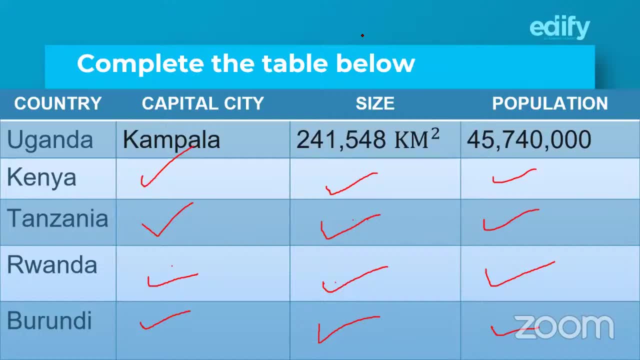 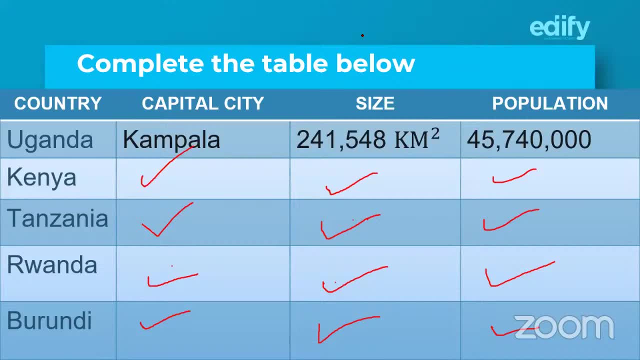 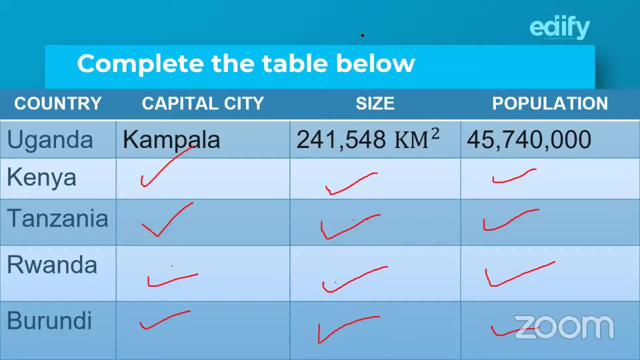 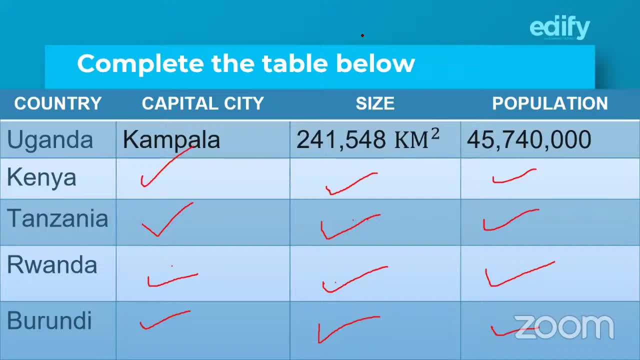 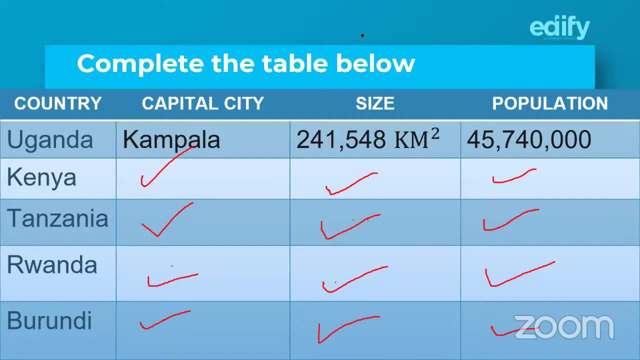 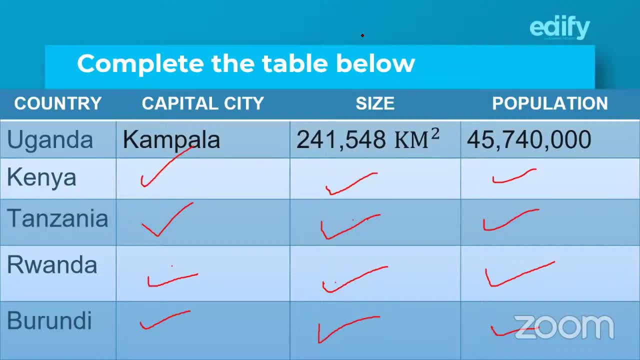 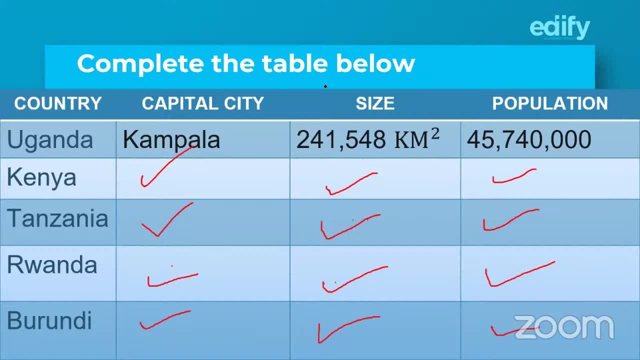 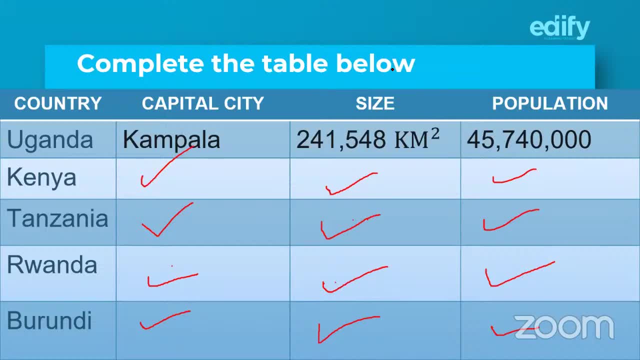 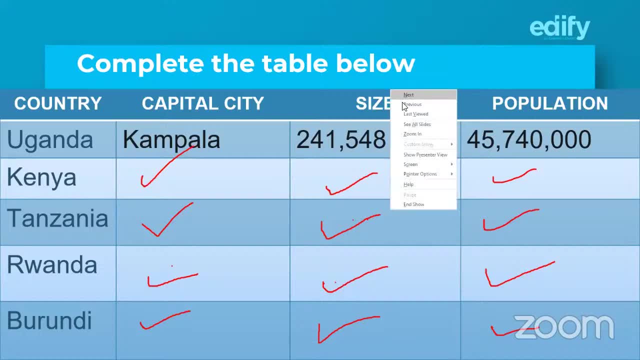 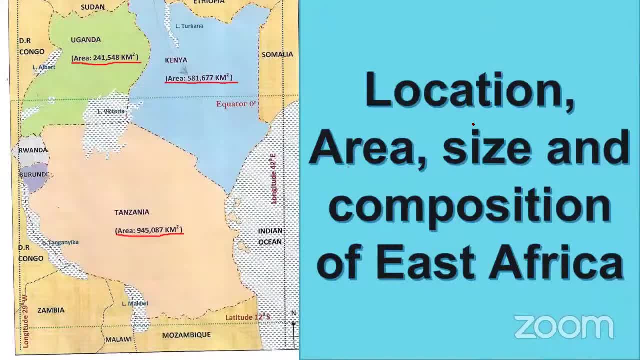 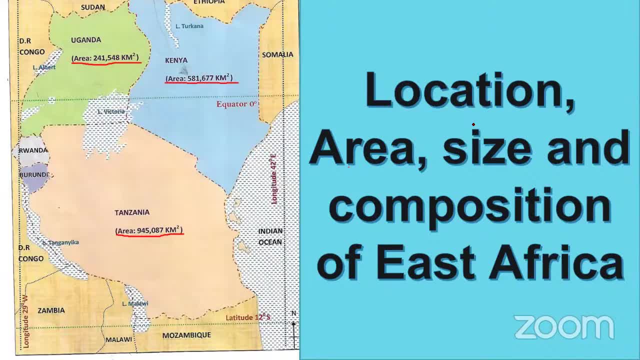 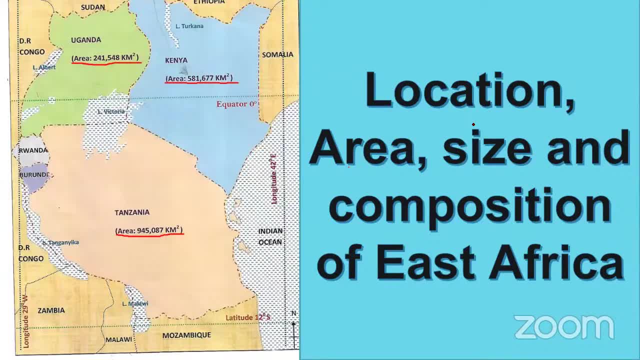 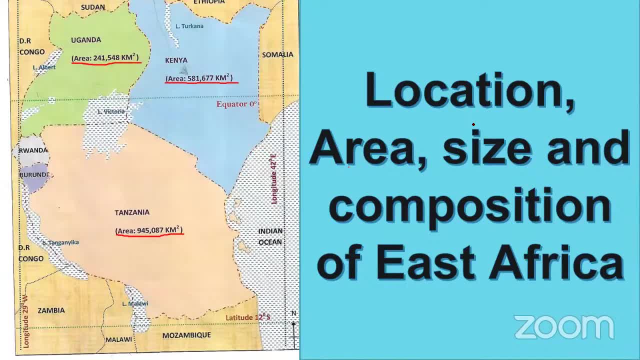 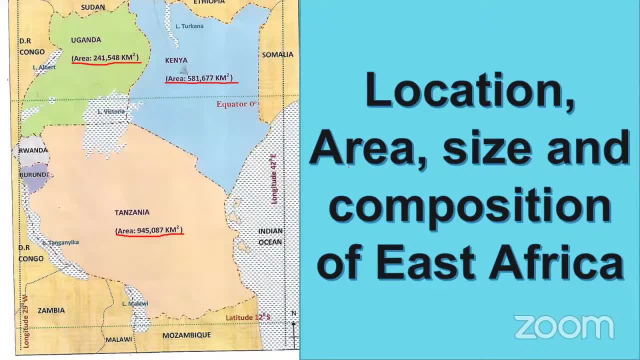 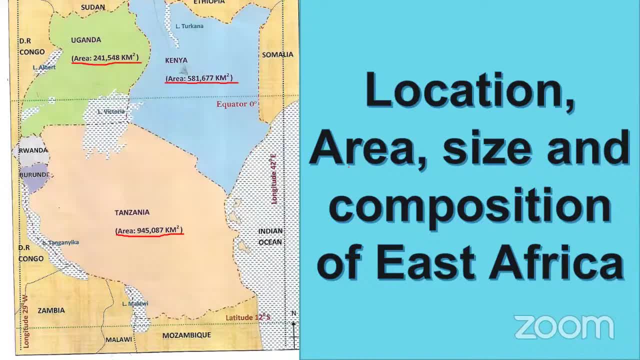 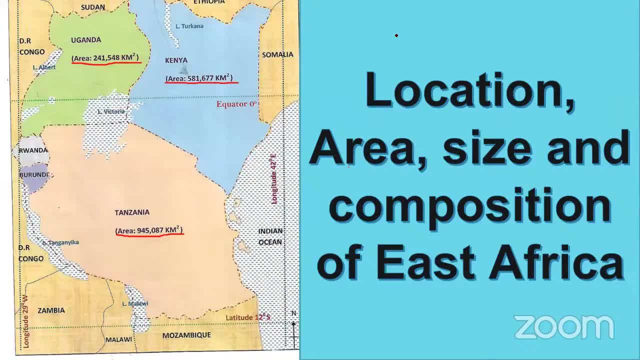 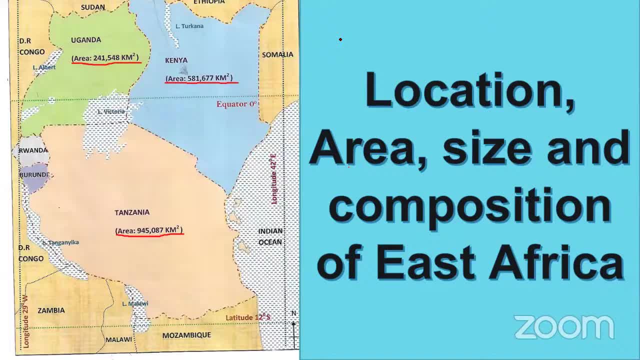 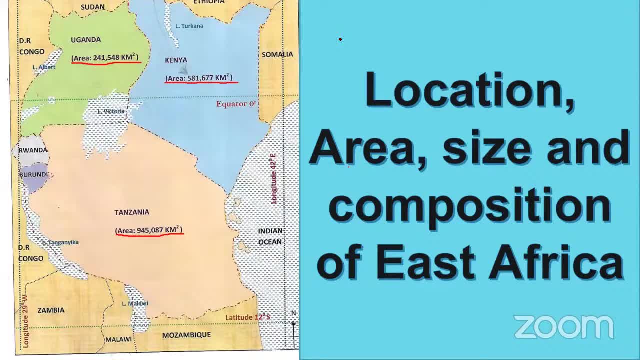 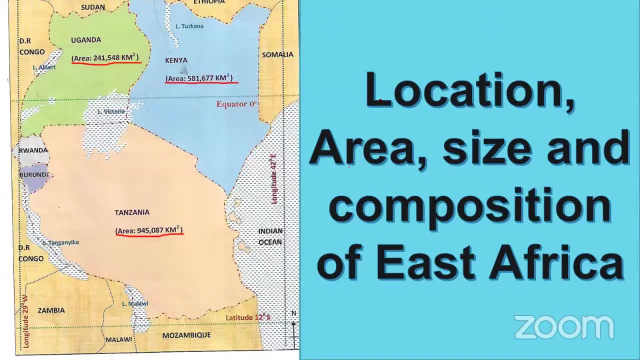 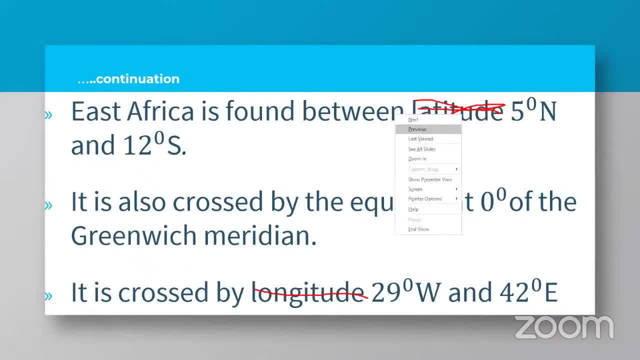 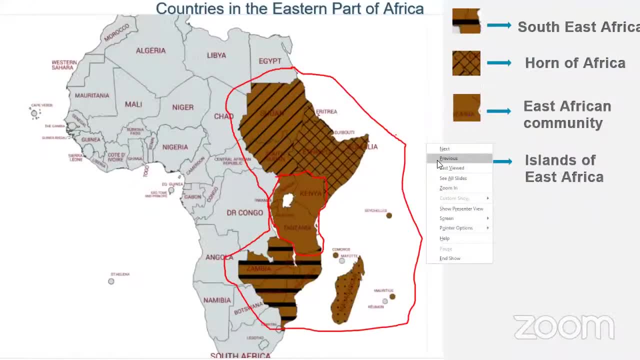 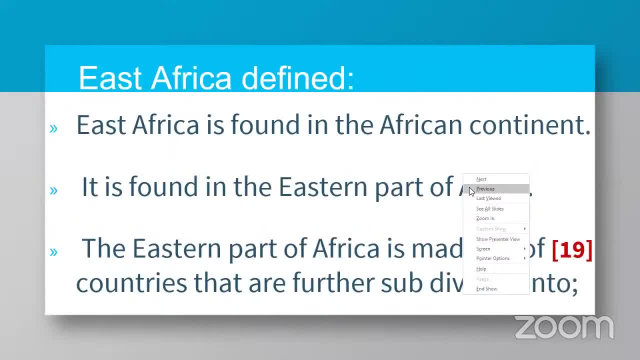 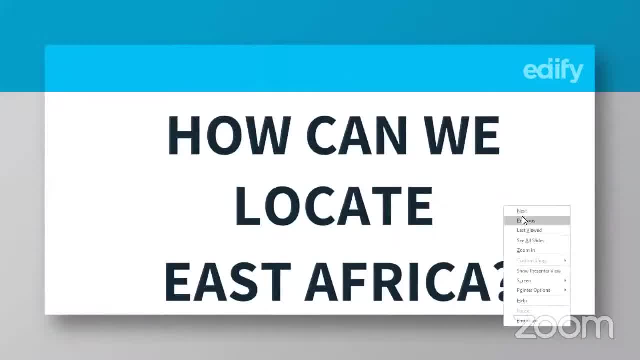 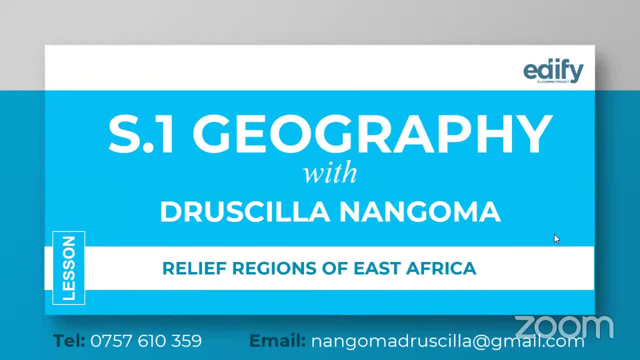 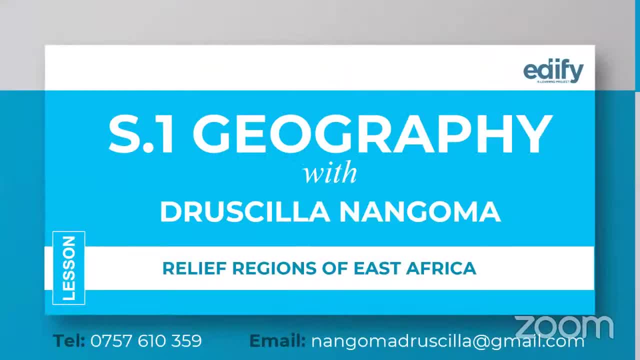 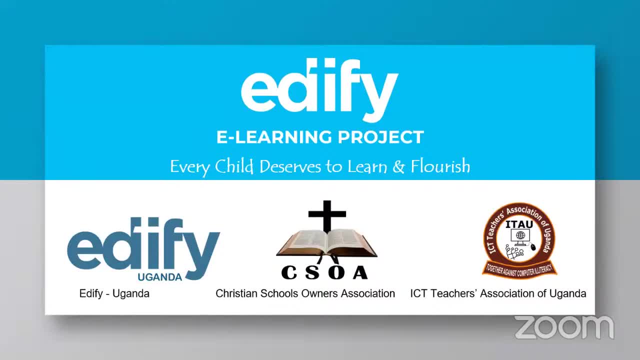 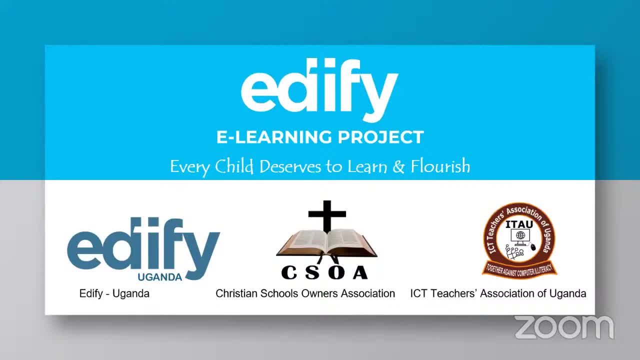 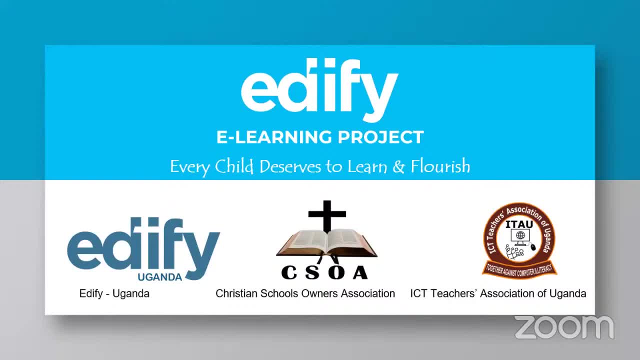 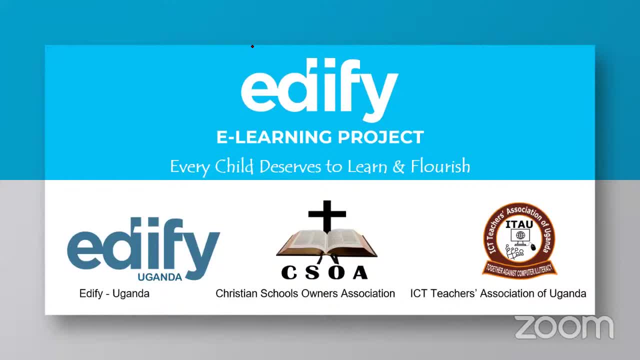 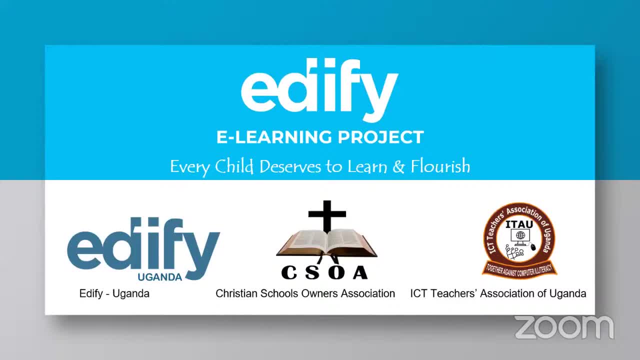